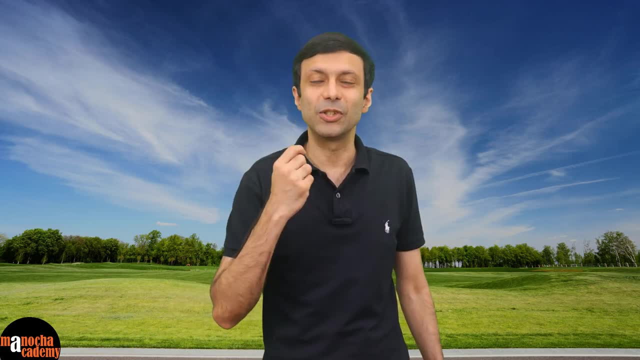 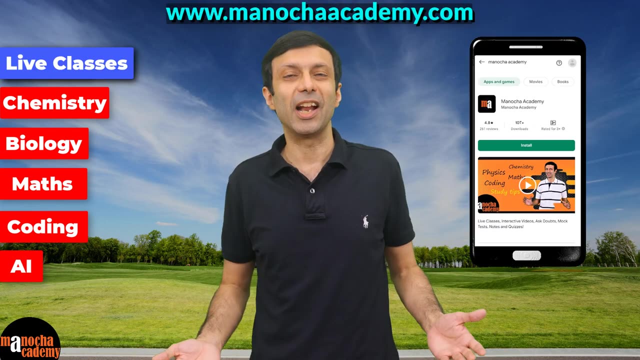 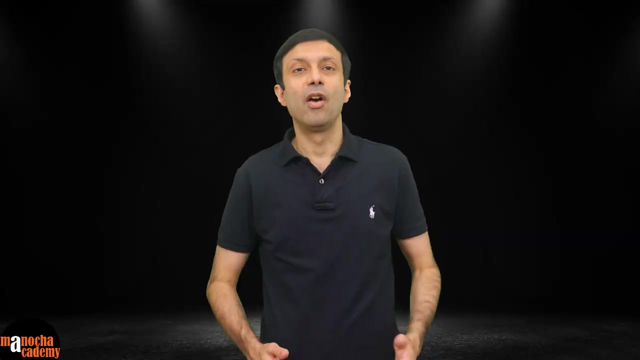 Now, before we begin, I would like to let you know that we have courses on science, maths, coding and artificial intelligence on our website and android app, So do check it out. The links are given below. Alright, let's get started and dive into the world of vectors. 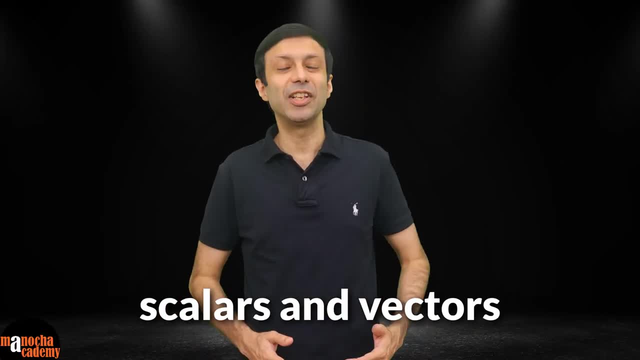 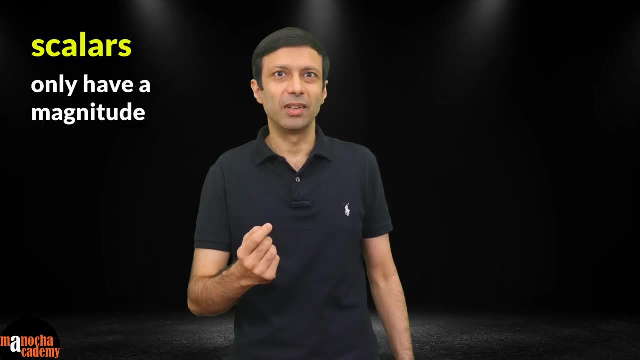 First let's talk about scalars and vectors and see the difference between these two. Scalar quantities are those physical quantities which only have a magnitude, They only have a value but no direction. Example of scalars are mass, distance, time, temperature, etc. 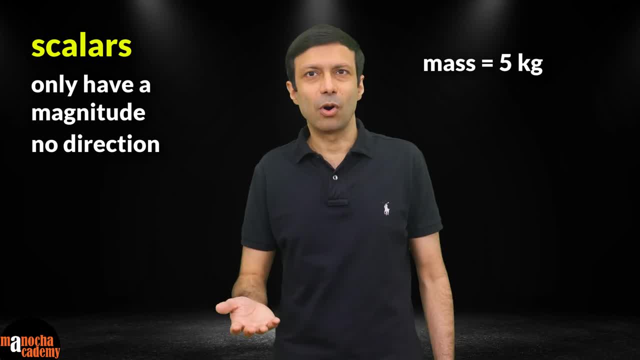 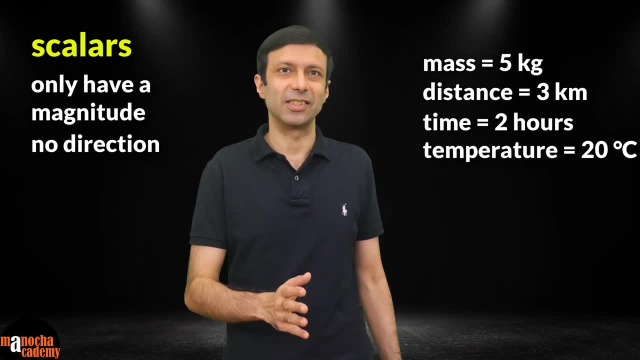 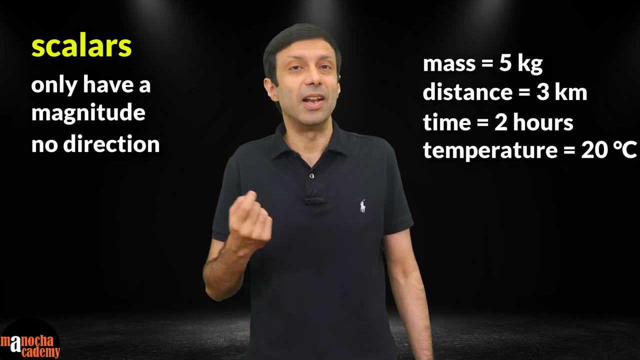 For example, we can say mass equals 5 kg, or distance equals 3 km, or time is 2 hours, or the temperature is 20 degrees Celsius. These are all scalar quantities. They only have a magnitude that is specified by the number here and the units. 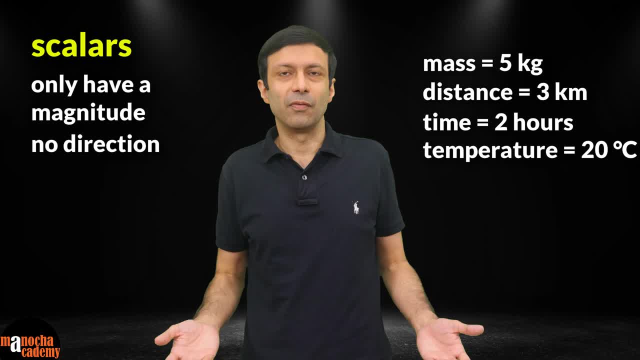 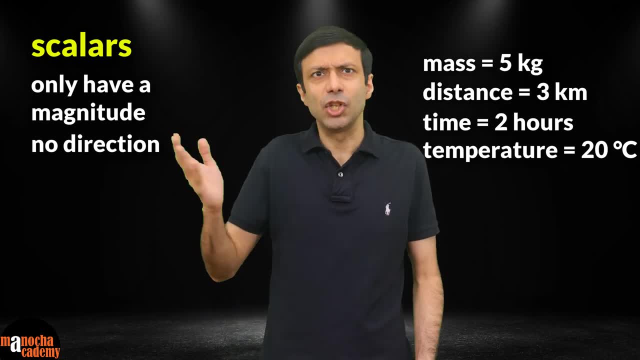 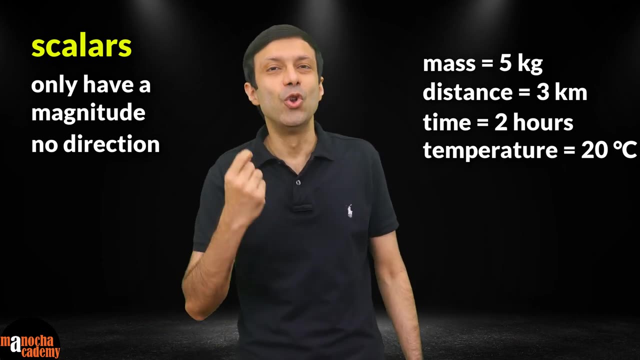 But they don't have any direction. When you say mass equals 5 kg, 5 kg is the magnitude, the value. We don't say 5 kg north or 5 kg south. That doesn't make any sense because it is a scalar quantity. It has no direction, only a magnitude. 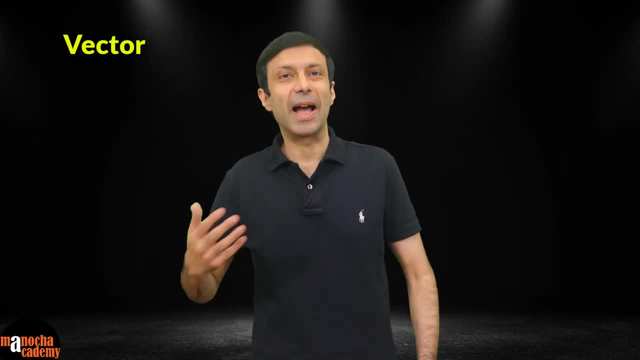 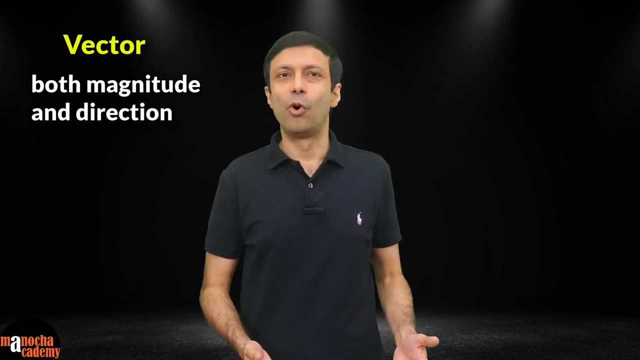 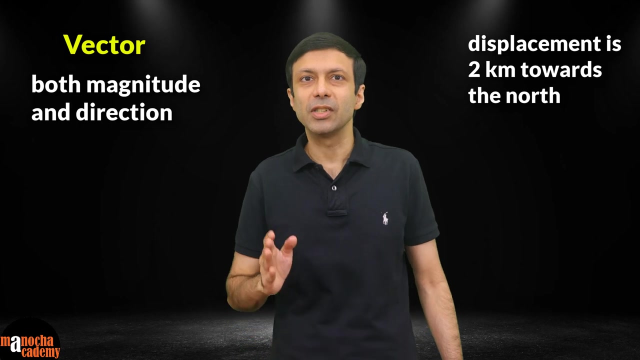 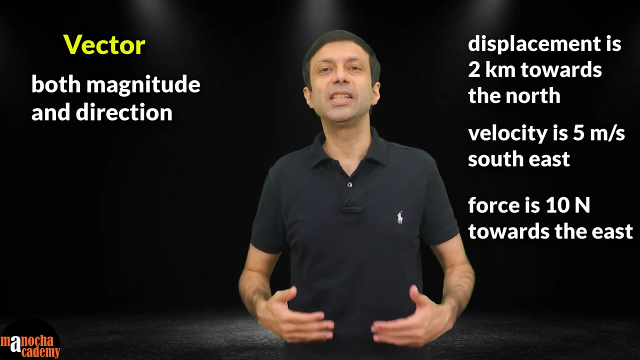 Vector quantities are those physical quantities that have both magnitude and direction. Examples of vectors are displacement, velocity, force, momentum and so on. For example, we say that the displacement is 2 km towards the north, or velocity is 5 m per second southeast, or force is 10 N towards the east, 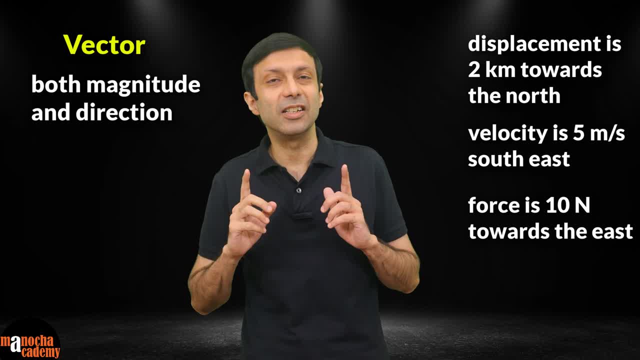 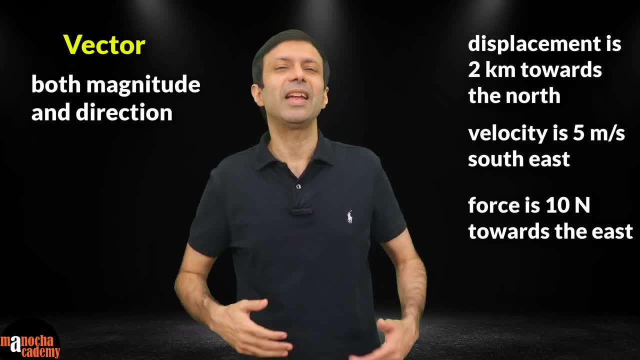 Vectors have a magnitude, They have a value and a direction. Sometimes, when we say that the force is 10 N, we are specifying the magnitude But we are ignoring the direction here. But this does not mean that force does not have a direction. 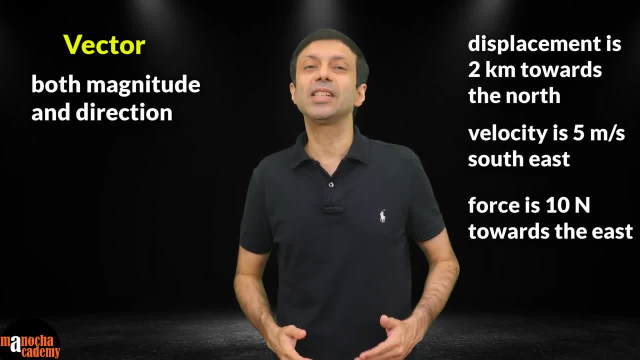 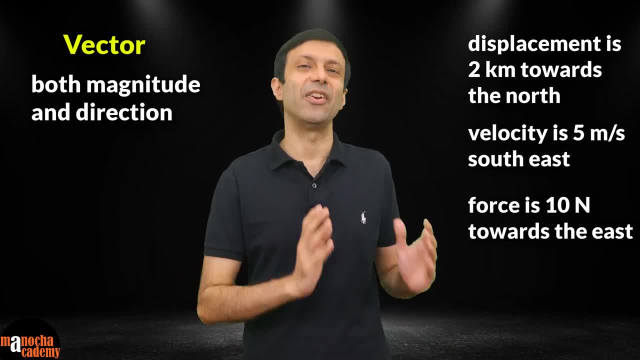 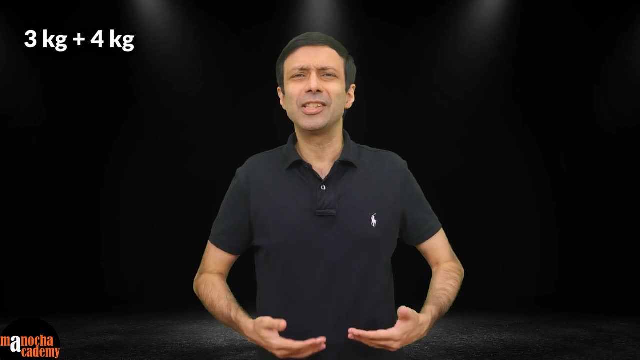 Force is a vector quantity. It has a direction. We just haven't specified it. So remember: vector quantities both have a magnitude and a direction. Let me ask you a question: What is 3 kg plus 4 kg? You will say it so simple: it is 7 kg. 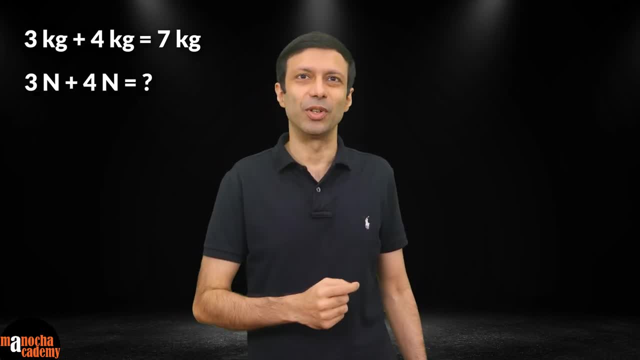 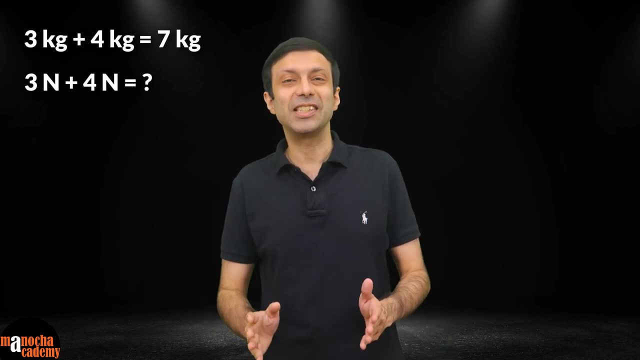 Now let me ask you What is 4 kg plus 4 kg? That is the vector quantity. You can simply 3N plus 4N. Is it 7N? This is true only in the special case where the two forces are in the same. 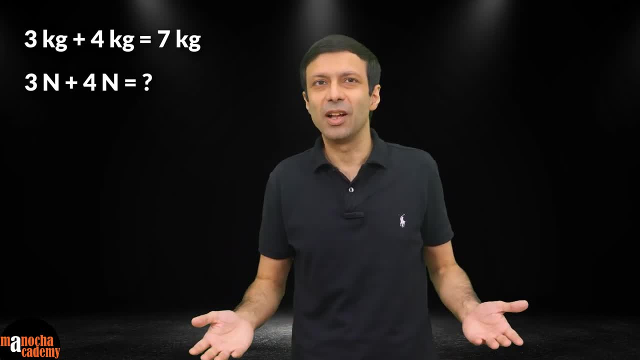 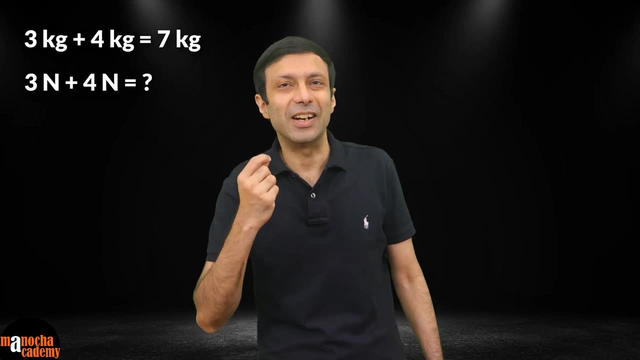 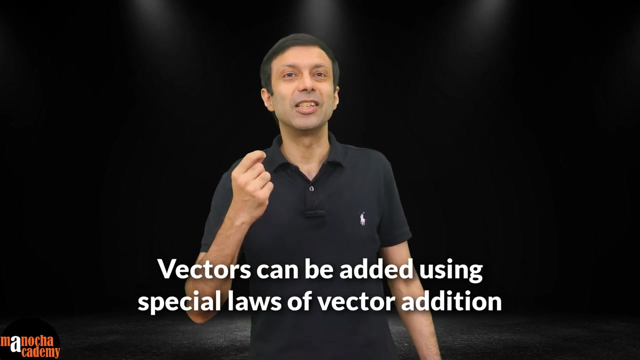 direction. If the two forces are in different directions, we can't simply do 3N plus 4N equal to 7N. We need to use vector addition. Scalers can be added according to the laws of algebra, but vectors need to be added using the special laws of vector addition. So remember: 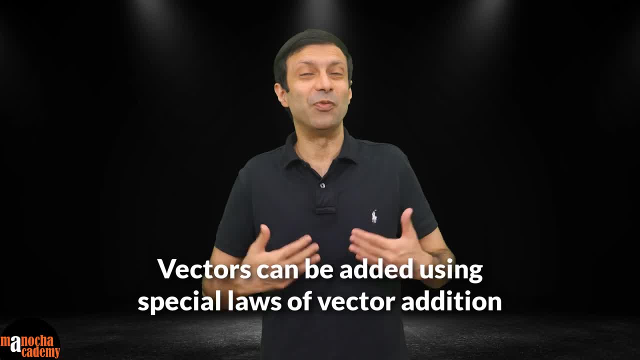 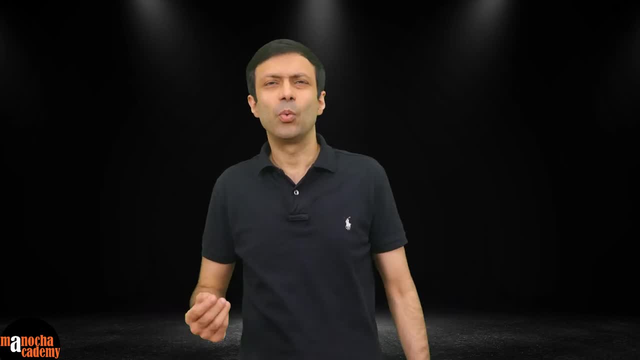 scalar and vector addition is not the same because these vector guys are different. They have a direction. Since vectors are different from scalars, we need a special vector notation to represent them. For example, force is a vector quantity. If we want to represent the force vector, 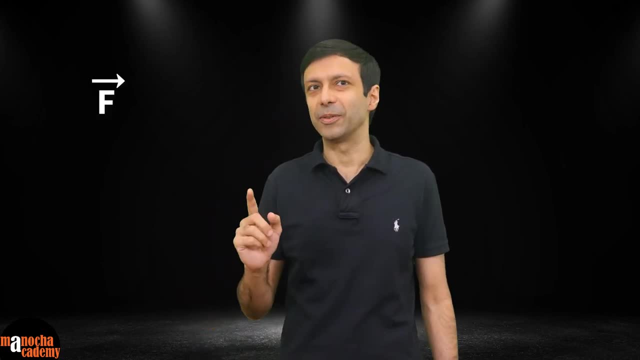 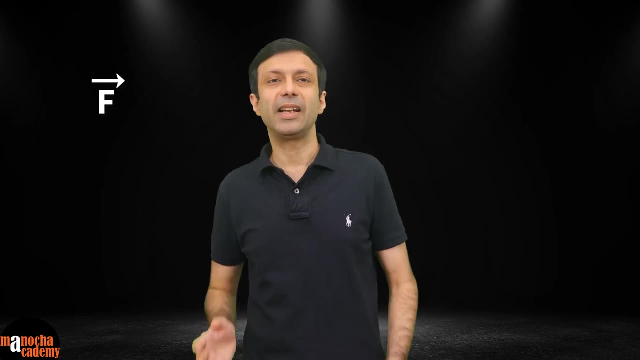 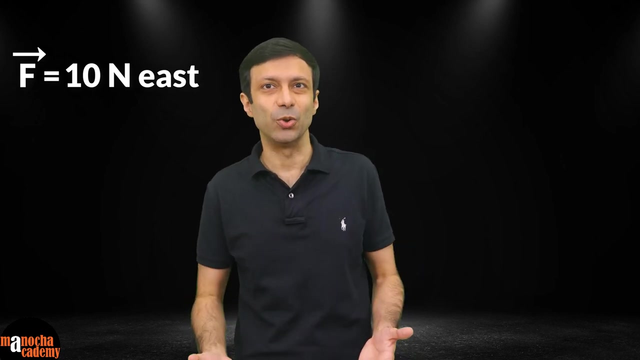 we write it as F with an F. F is written in bold to represent that it's a vector. For example, we can write F equal to 10N east. This represents the force vector of magnitude 10N and the force is in the east. 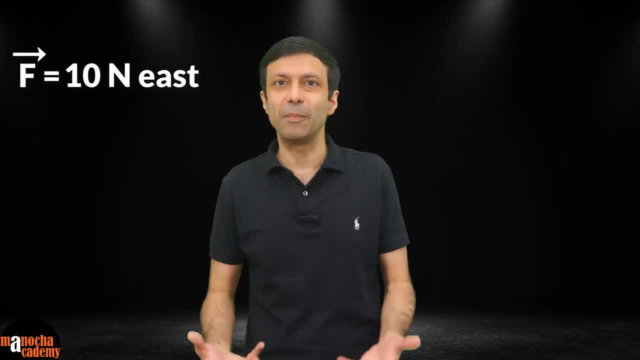 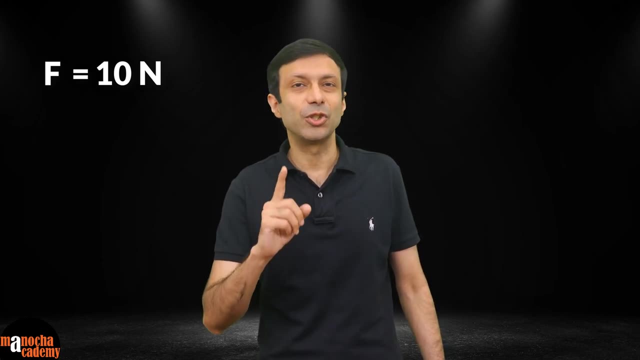 direction. Now, if we want to represent only the magnitude of the force vector, then we can write F equal to 10N. Note now that F does not have an arrow over it or it is not a vector. So if we want to represent only the magnitude of the force vector, then we can. write F equal to 10N. Now if we don't want to represent only the number of jardins on a vector, F can represent only a number of jardins. that is a vector as the short address. So if we want to represent only the magnitude of the force vector, that is a a. 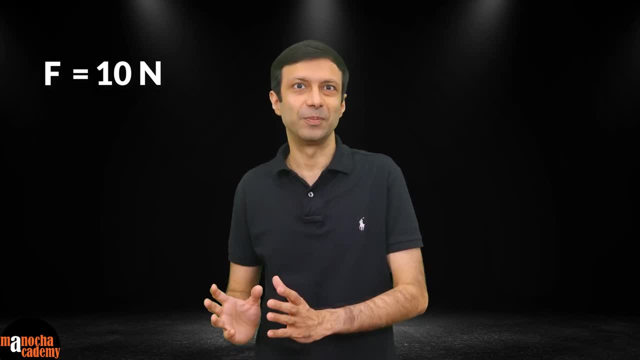 vector, then we can write F equal to 10N. Note now that F is represented only in bold. So we are representing magnitude. So say we have this P. Another way to represent the magnitude is by drawing two vertical lines around F. So 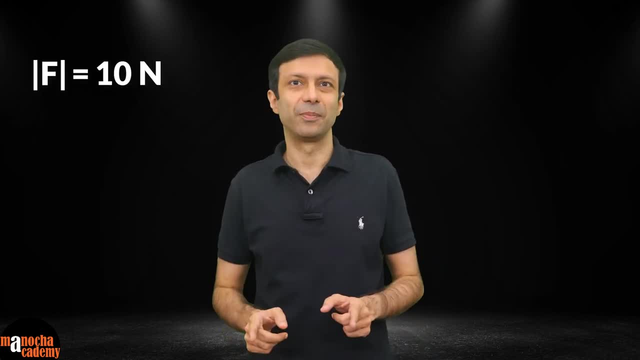 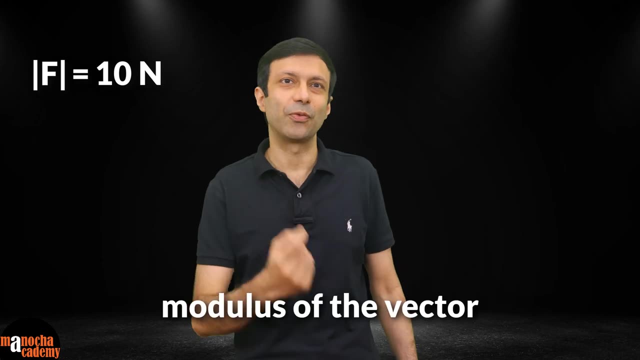 So it gives us F equal to 10N. This is also called the modulus for the vector, So this f is theienda f, ethics a, the magnitude of the force vector without it's direction, So it's only the value of the vector. and those vectors can also be represented visually. 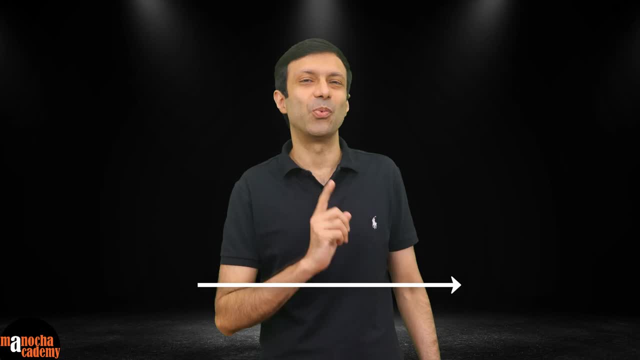 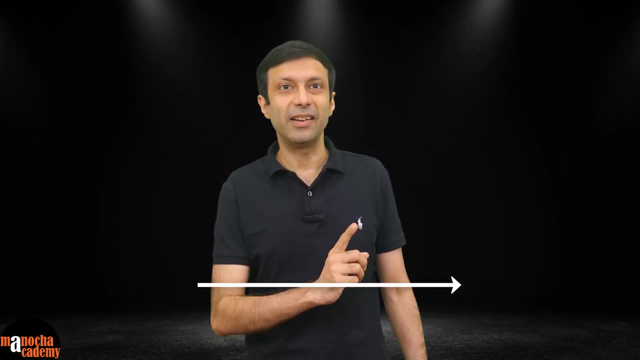 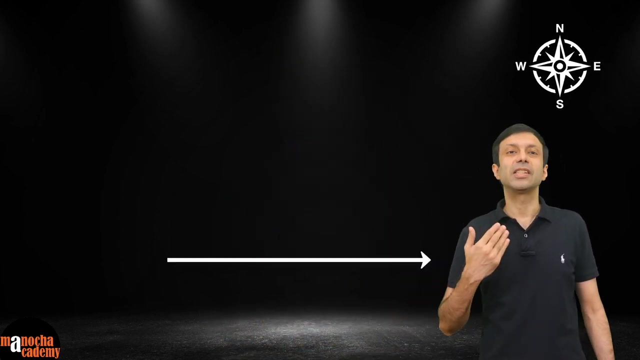 by drawing a straight line with an arrowhead at one end. The length of the line gives you the magnitude of the vector and the arrowhead gives you the direction. For example, this vector drawn here represents a force of 10 Newton towards the east, and this vector represents 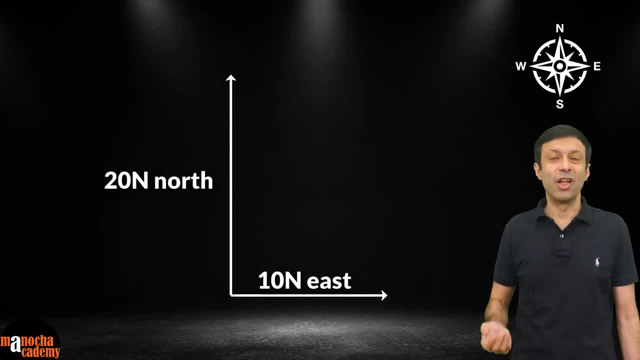 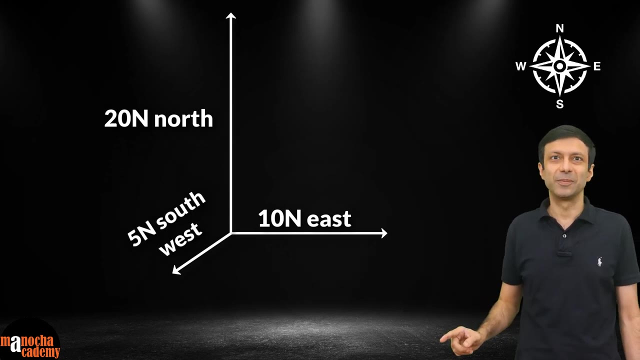 a force of 20 Newton towards the north. Note that it is double in length compared to the 10 Newton force vector and it points towards the north. And this vector represents a force of 5 Newton towards the south-west. Note that it is half in length compared to the 10 Newton. 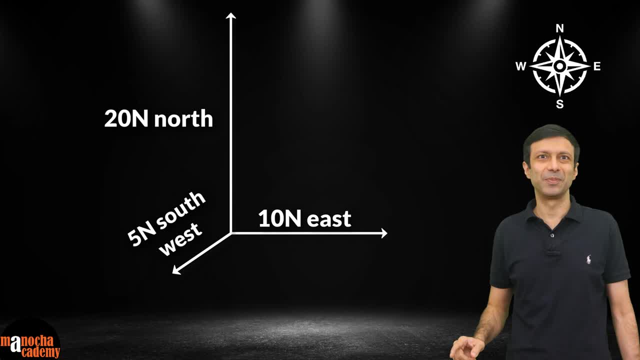 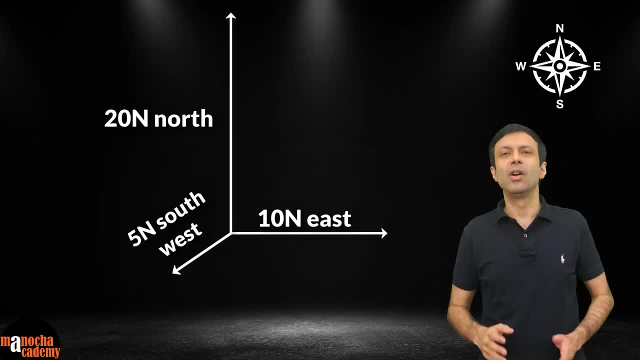 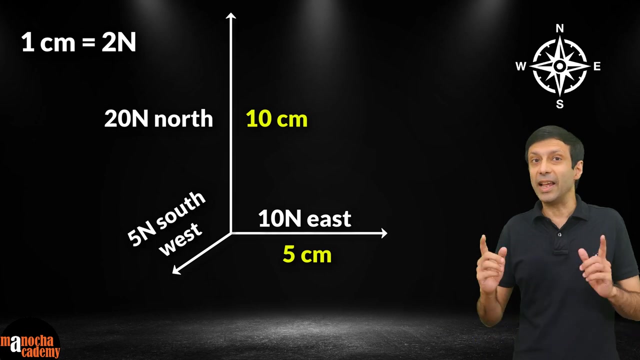 vector and it's pointing towards the south-west. So, just like in coordinate geometry, we use a scale for the length of the vector, For example 1 cm. here is 2 Newton, So a 10 Newton vector can be represented by a line of length 5 cm. For 20 Newton we will use a line of 10 cm and so on. So the 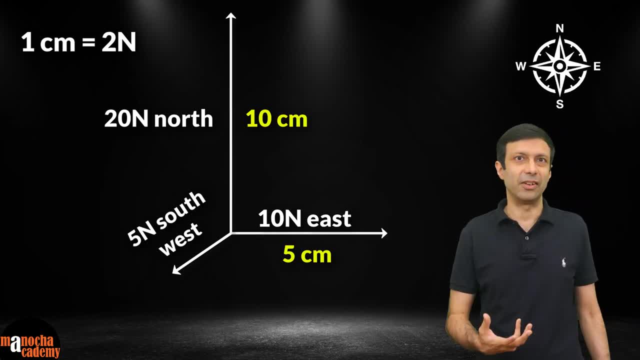 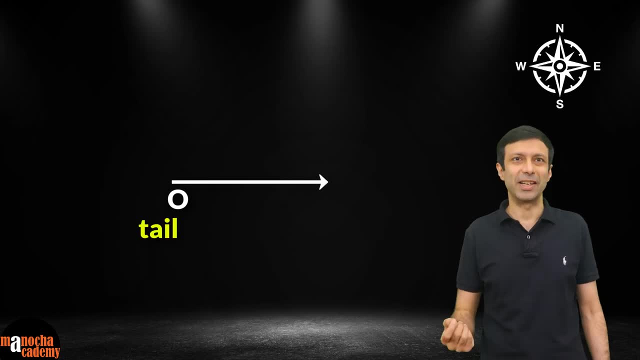 length of the line is indicating how large the vector is. The starting point of the vector, represented by O, here is called the tail of the vector, and the ending point, represented by A, here is called the head of the vector. So the vector has a head and a tail, and the 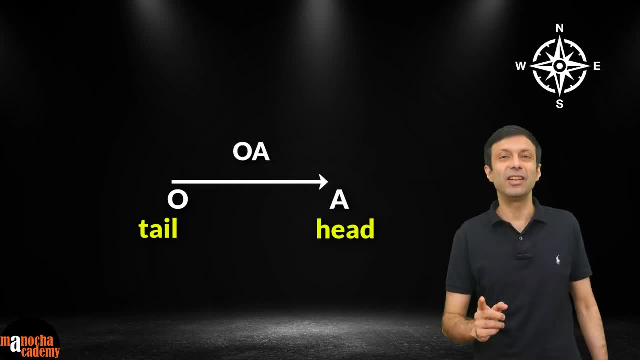 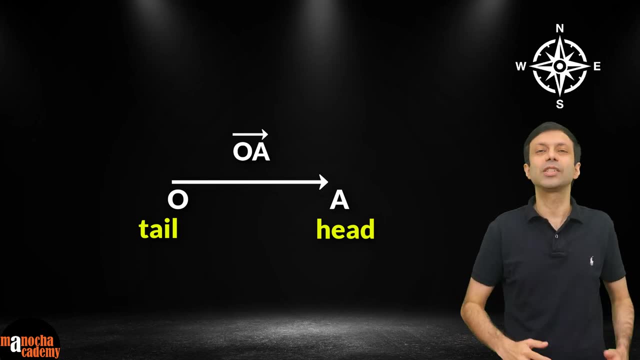 vector. here is OA, and it is written with an arrow on top of it. Remember the arrow represents that we are talking about a vector quantity, or sometimes you write OA in bold. These are both vector notations, right. So either you use the arrow or represent it in bold to indicate: 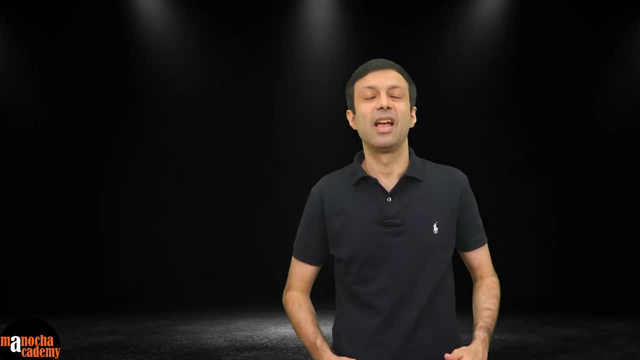 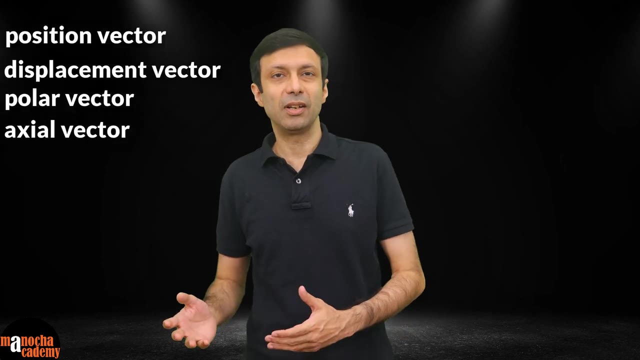 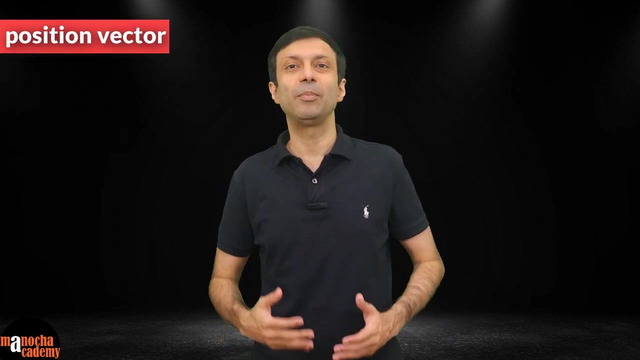 that we are talking about a vector quantity. Now you know the basic concept of vectors. let's discuss some important types of vectors, such as position and displacement vectors, and polar and axial vectors. A position vector is used to describe the location or position of a point or object. 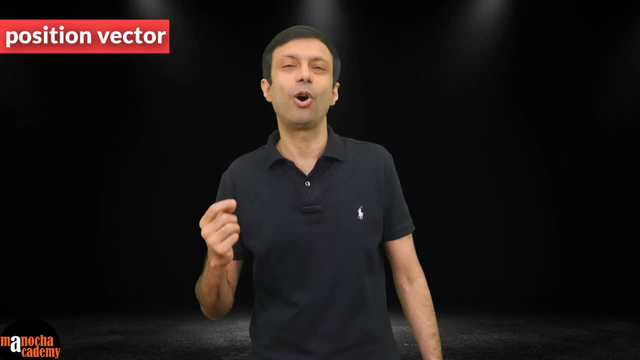 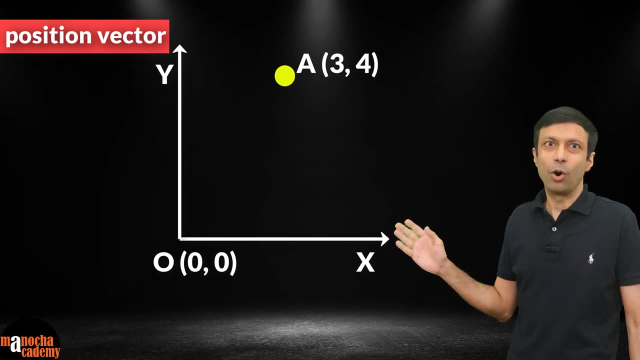 in space relative to a chosen reference point or origin. For example, let's say an object A is located at 3,4 here on the coordinate plane, Then the vector drawn from the origin O, that is 0,0 to A 3,4, is called the position vector. 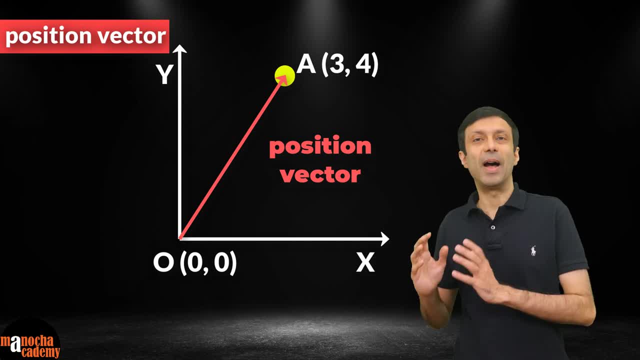 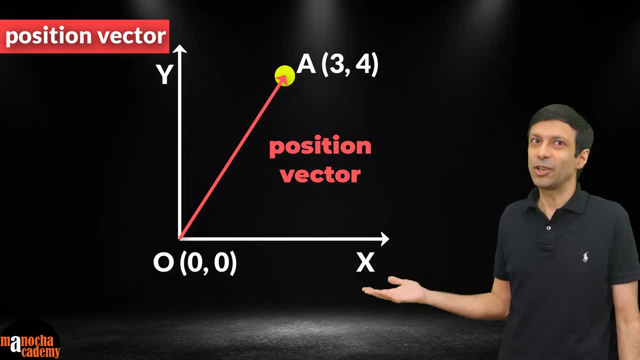 of the object Position vector has both magnitude and direction. Now, what is the magnitude of the position vector OA here? Can you calculate it? That's right. Let's use Pythagoras theorem and calculate the magnitude or the length of the vector. 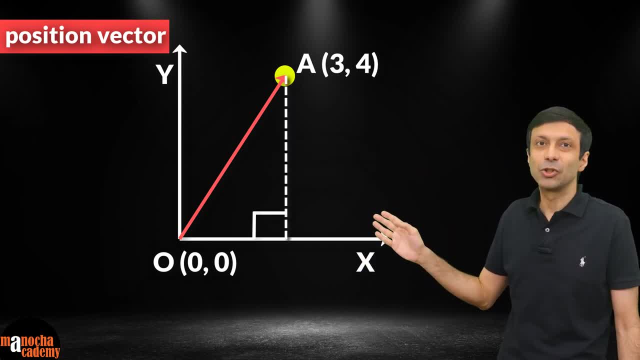 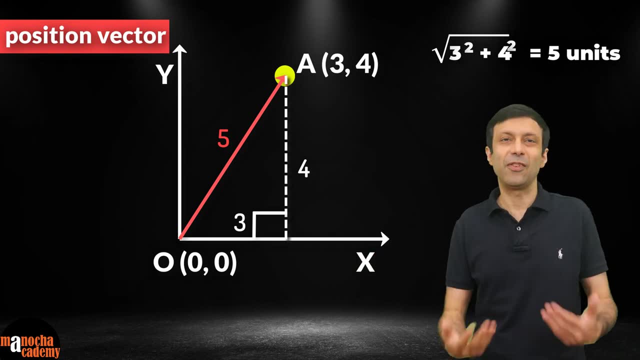 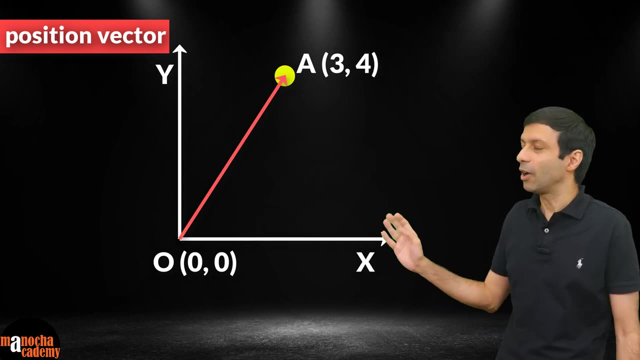 Since we have a right angle triangle here. so the length of the vector is going to be the hypotenuse, which is going to be square root, of 3 square plus 4 square, which equals 5 units. So OA has a magnitude of 5 units and the direction of this vector is roughly towards the northeast. 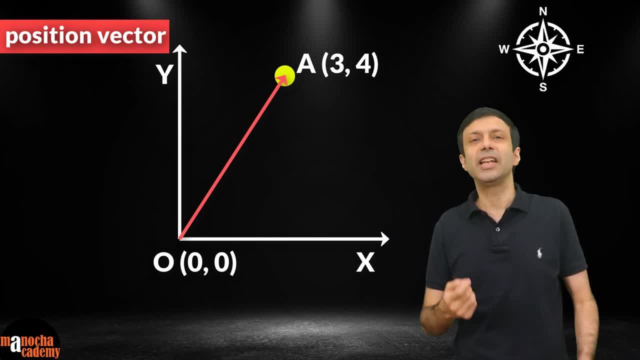 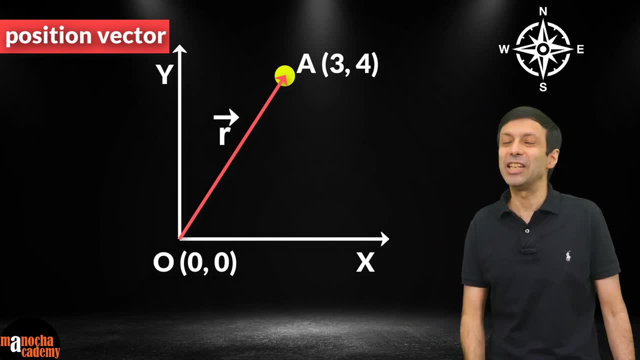 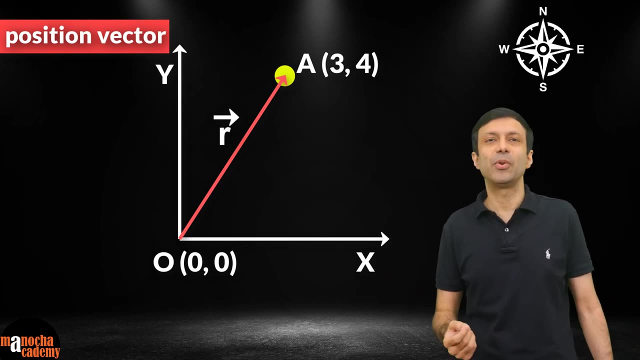 direction you can see here. Now, the position vector is often denoted by r with an arrow on top of it, or r written in bold, and its job is to give the position of the object. Now, mathematically, this position vector can be represented as r equal to 3i plus 4j, where 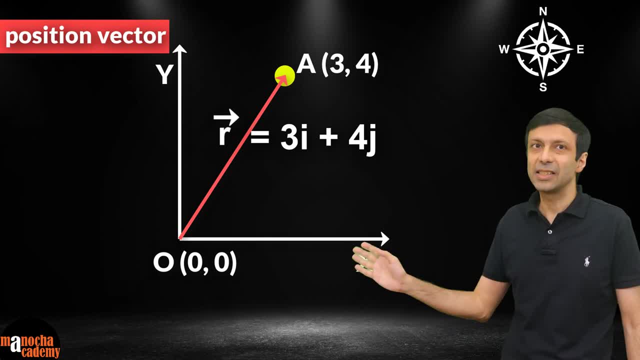 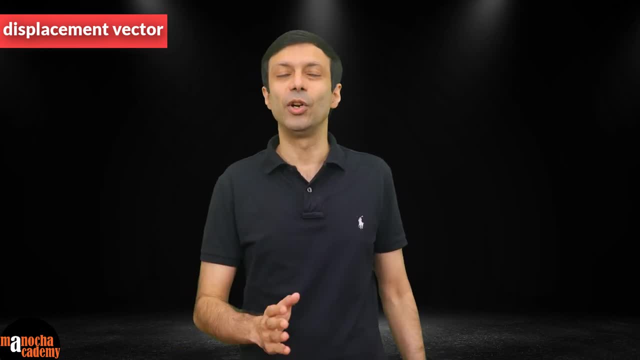 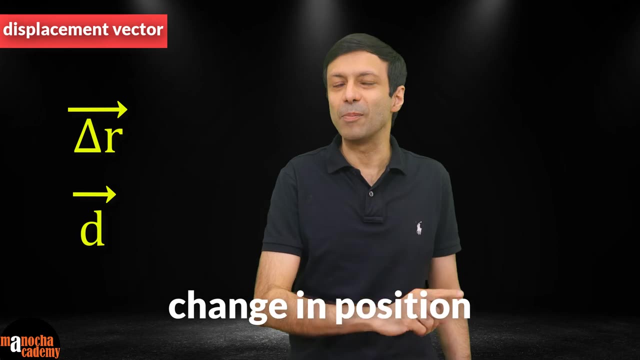 i and j are the unit vectors along the x and y direction. Next, let's look at the displacement vector. A displacement vector is often denoted as delta r. Delta r represents the change in position of an object as it moves from one point to. 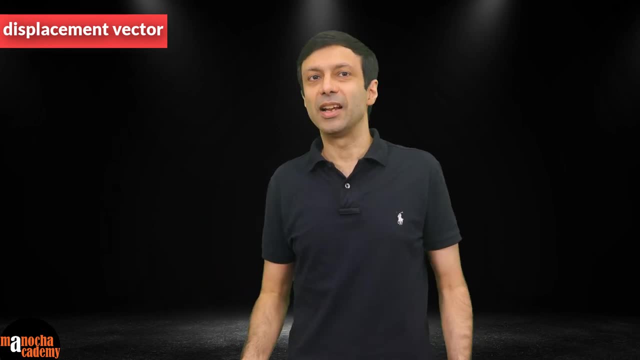 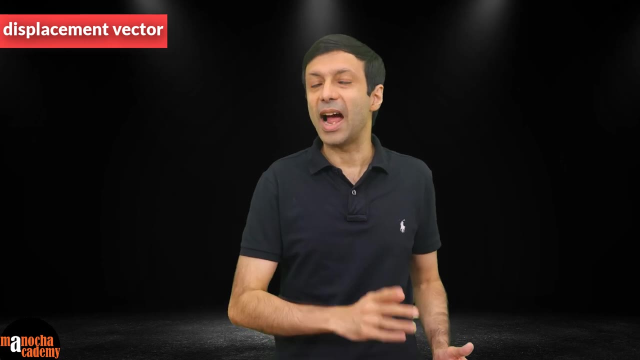 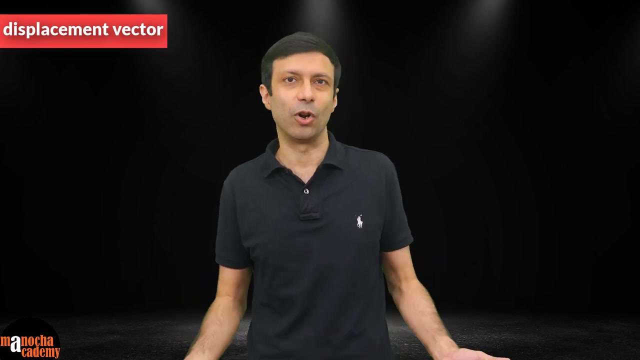 another in space. Like position vectors, displacement vectors also have both magnitude and direction, indicating how far and in which direction an object has moved. Displacement vectors are not concerned with the path taken by an object. they only describe the change in position from the initial to the final. 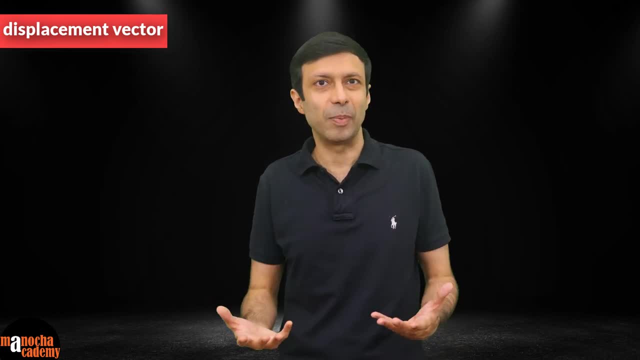 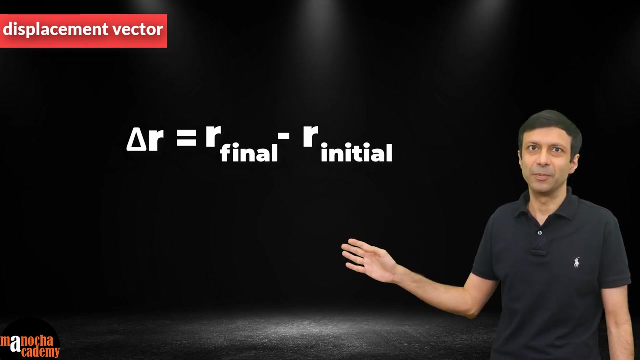 Because, remember, that is the definition of displacement- the shortest distance from initial to the final point. Now, mathematically, the displacement vector can be found by subtracting the initial position vector from the final position vector. So we can write delta r equal to r final minus r initial. 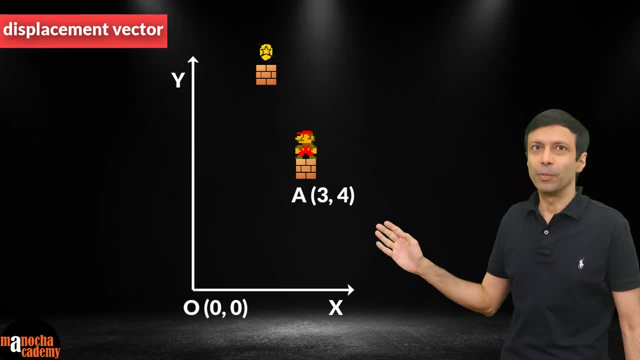 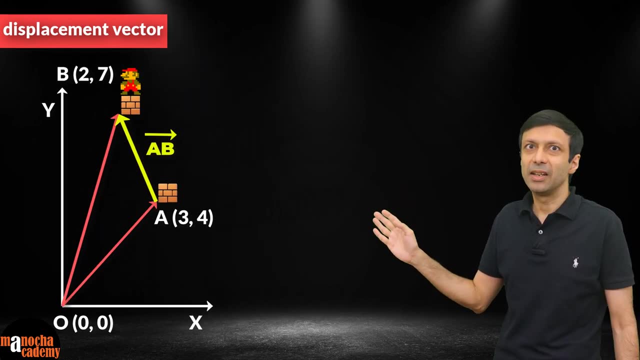 For example, if the object was initially at 3 comma 4. And let's say it moved to b, Then the displacement vector ab is going to be 2i plus 7j minus 3i plus 4j. So you subtract the initial position vector from the final position vector. 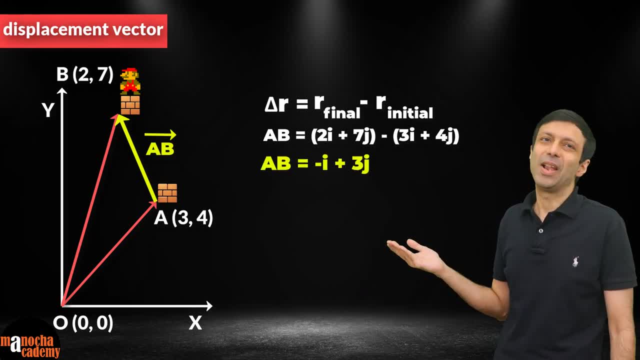 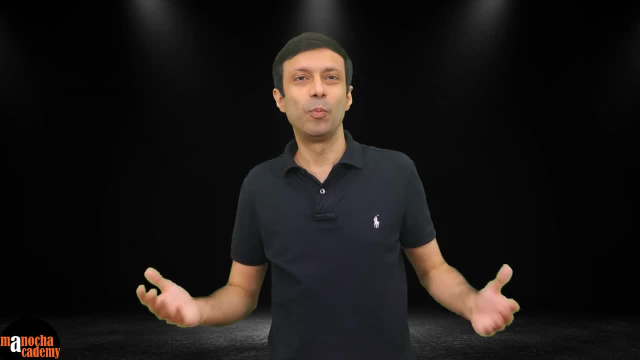 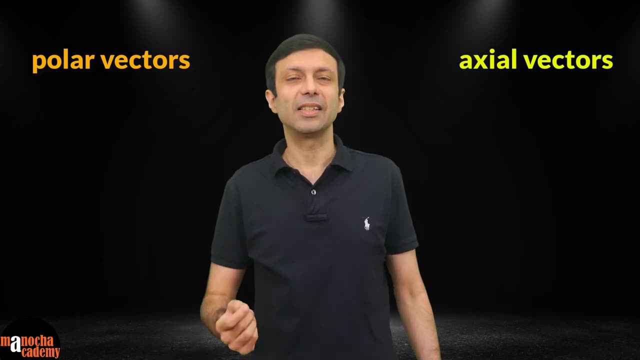 And we get the answer minus i plus 3j. So that is our displacement vector ab here. Vectors can be divided into two broad categories: Polar vectors And axial vectors. Polar vectors are those vectors that have a starting point or a point of application. 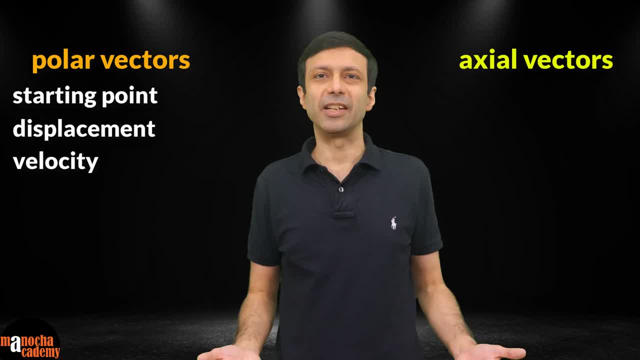 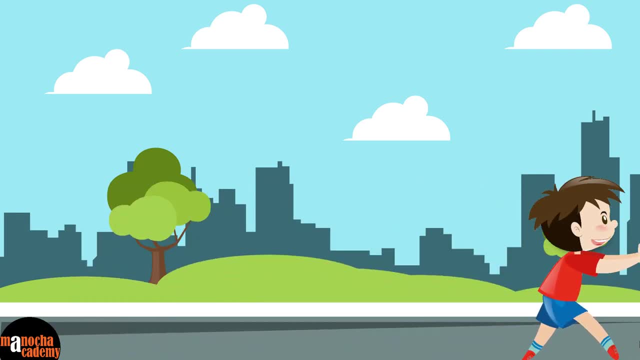 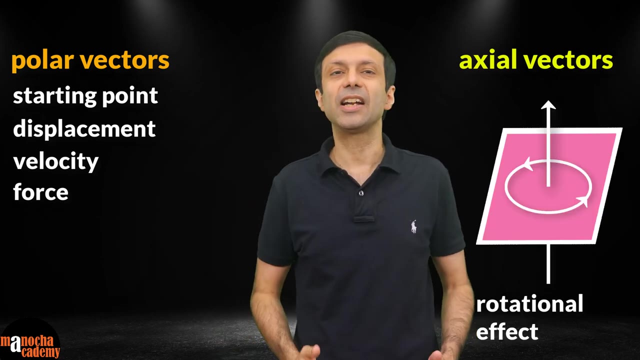 For example, displacement and velocity. these are polar vectors since they have a starting point. Force is also a polar vector since it has a point of application. Axial vectors are those vectors which represent a rotational effect and act along the axis of rotation. 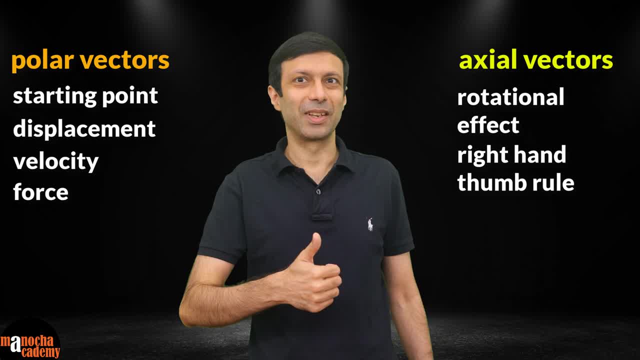 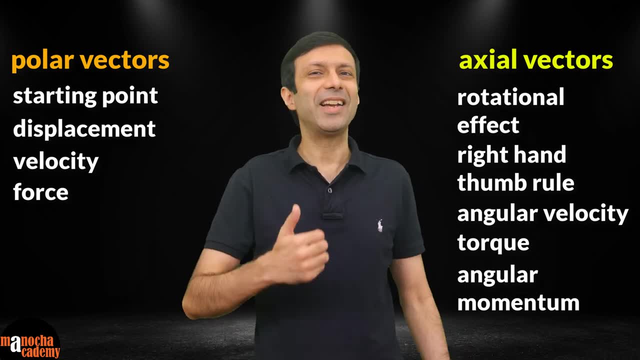 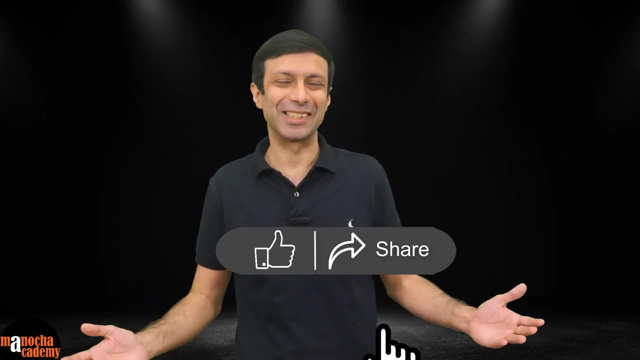 Based on the rotation. This is called the right hand thumb rule. Examples of axial vectors are angular velocity, torque and angular momentum. The right hand thumb rule for axial vectors reminds me that. do hit the like button and share this video with your friends. 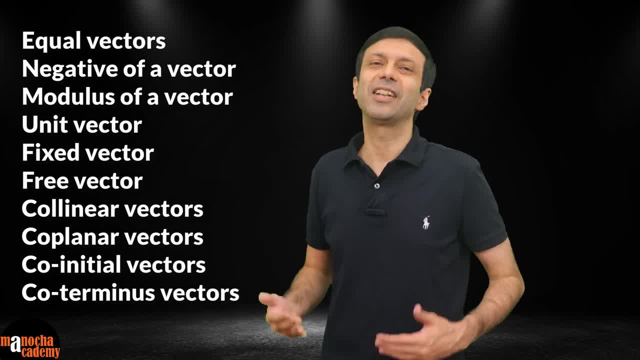 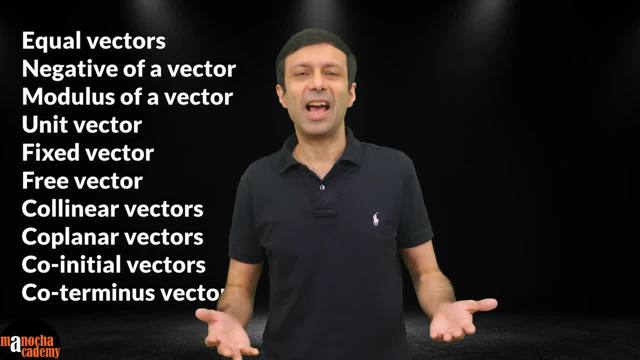 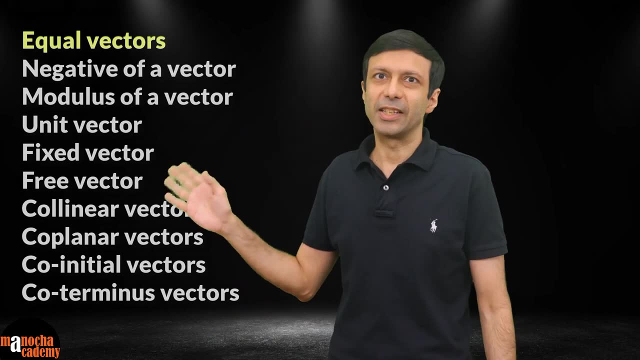 Now we will discuss some more important terms that are used in vector algebra. I know there are a lot of terms for vectors, but don't worry, these are simple and I will explain it with some examples. Let's start. We will start with equal vectors. 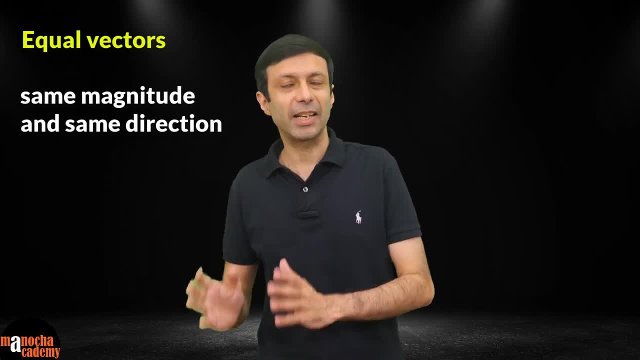 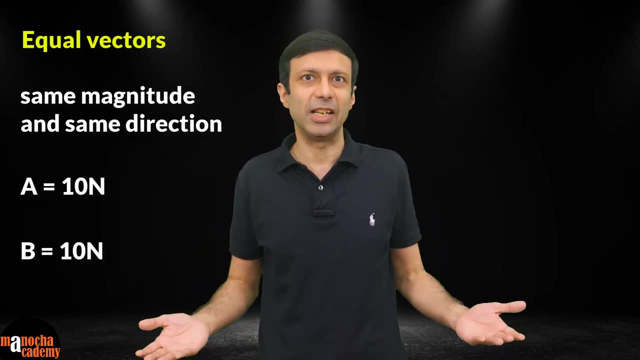 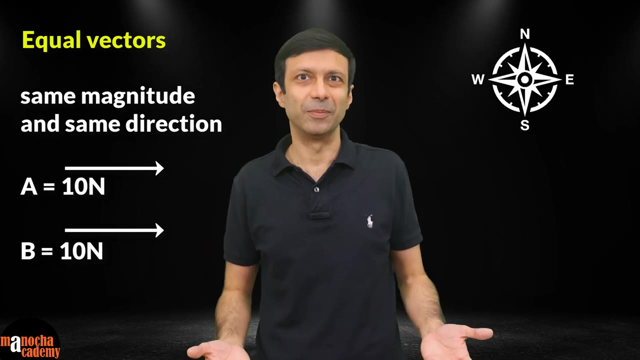 Two vectors are said to be equal if they have the same magnitude and the same direction. For example, if two force vectors are both 10 Newton each, and let's say both of them are acting towards the east direction, Then the two vectors are equal. 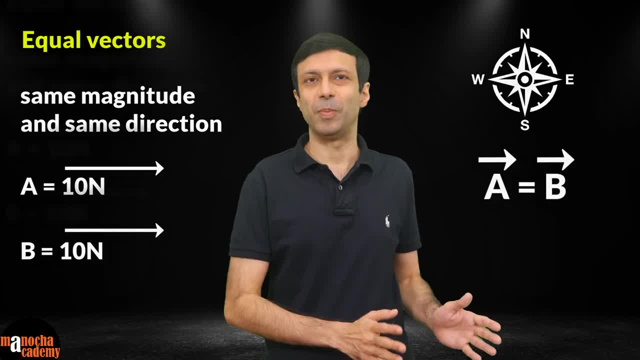 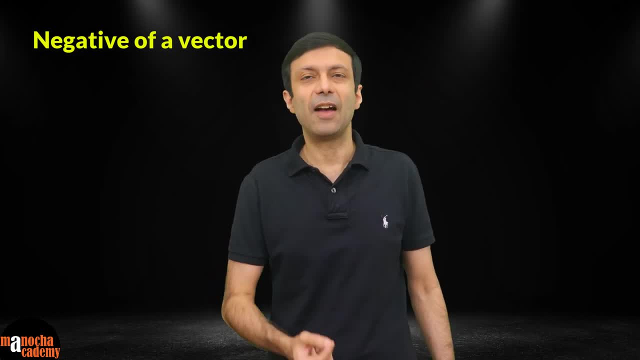 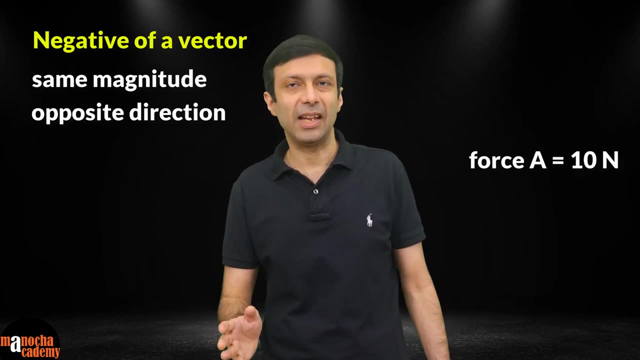 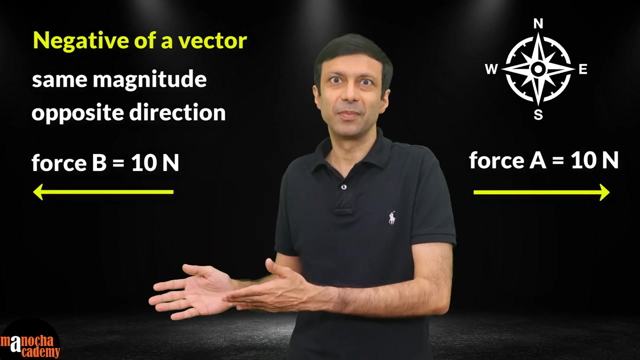 So we can write: vector a is equal to vector b. Now what is negative of a vector? Negative of a vector is another vector having the same magnitude but the opposite direction. So, for example, if there is a force A equal to 10 N towards the east and force B is 10 N towards the west, 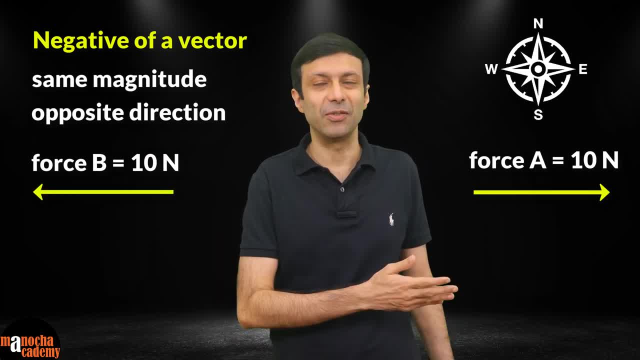 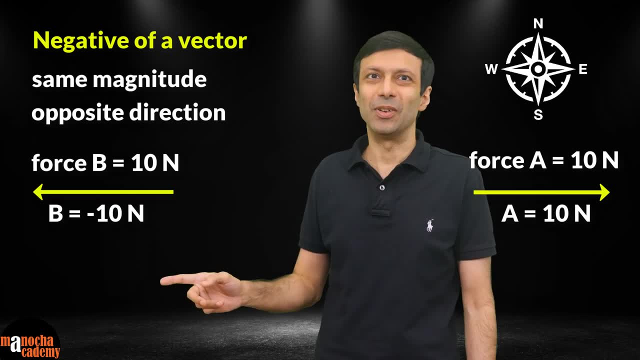 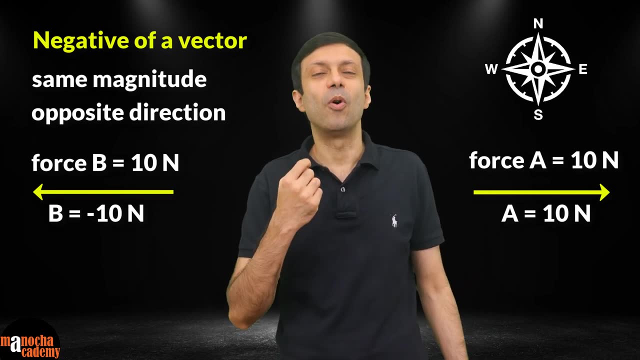 So if we take the direction towards the east as positive, we can write A equals 10 N. Then B is going to be written as minus 10 N because it's in the opposite direction. So according to vector notation we can write: B is equal to minus of A. 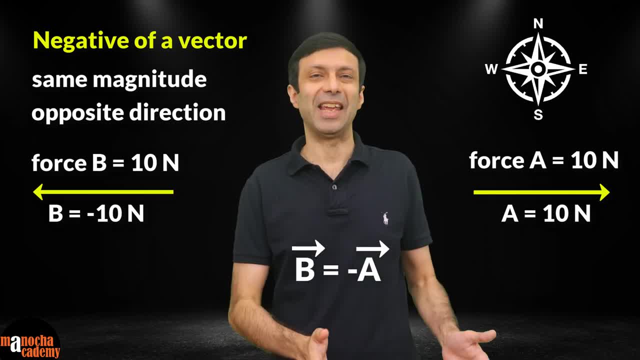 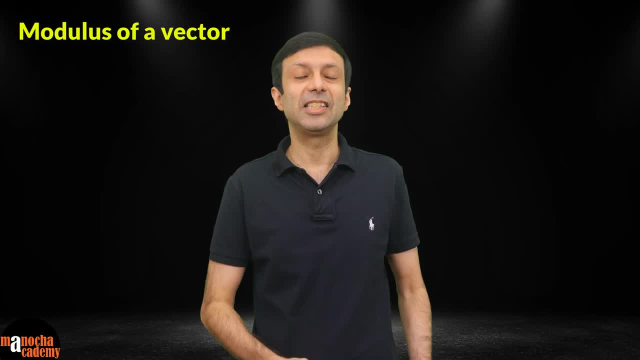 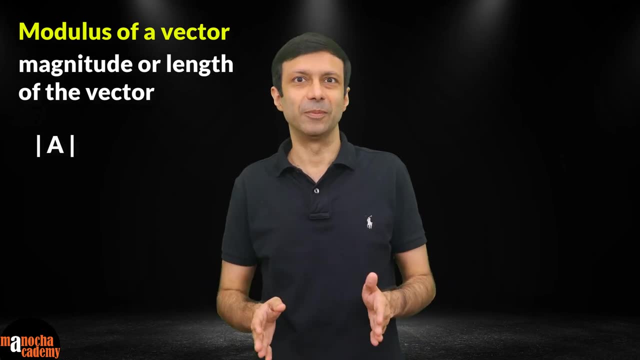 So B is the negative vector of A. here We have discussed modulus of a vector earlier. Remember, modulus of a vector is the magnitude or the length of the vector. We represent it by drawing vertical lines around the vector Or writing A without vector notation. 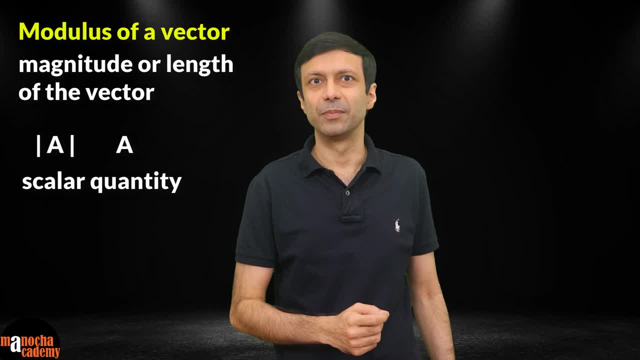 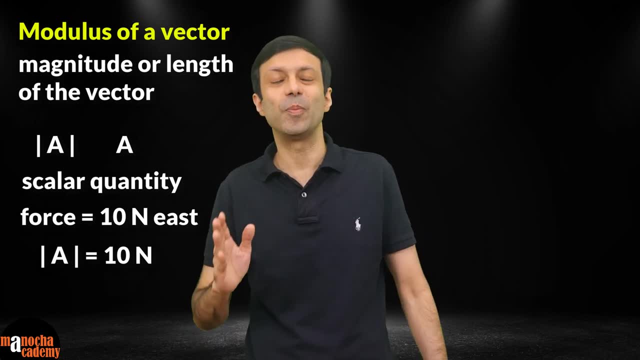 Magnitude or modulus is a scalar quantity. So for the force A equal to 10 N towards the east, the magnitude A is going to be equal to 10 N. That is just the value, without any direction. That is basically the modulus of the vector, only its magnitude. 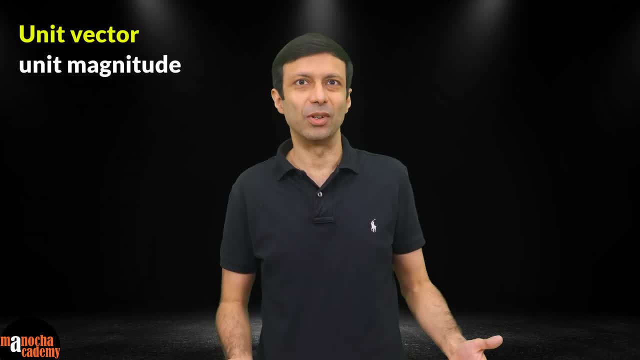 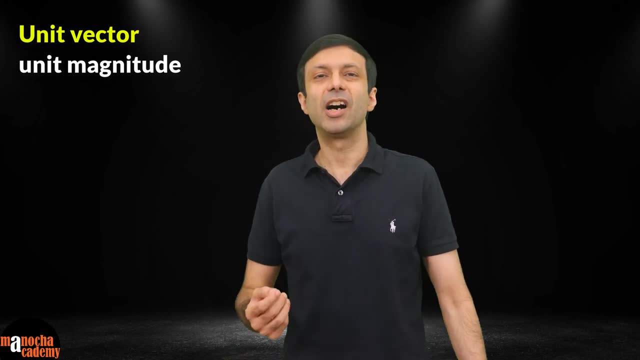 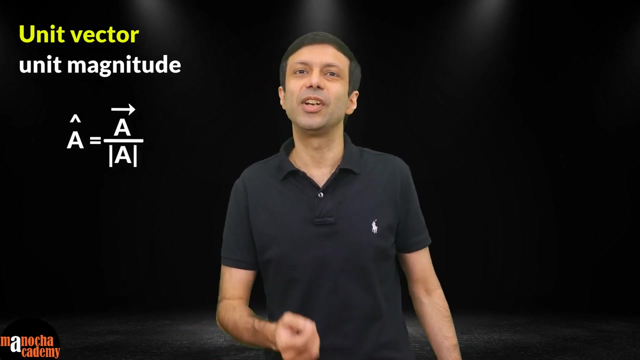 Unit vector is a vector of unit magnitude, Or we can say magnitude of 1. And it is drawn in the direction of the given vector. A unit vector can be obtained by dividing any vector with its magnitude. Unit vector is written with a caret symbol on top of it, as shown here. 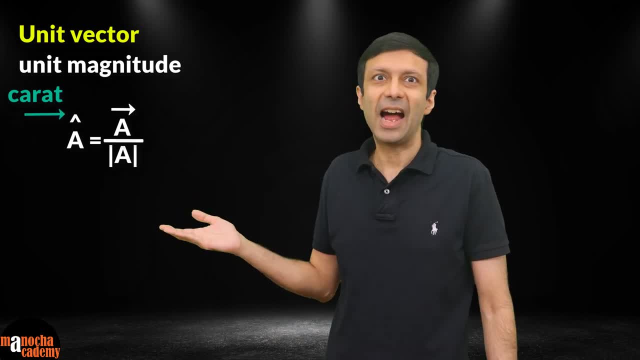 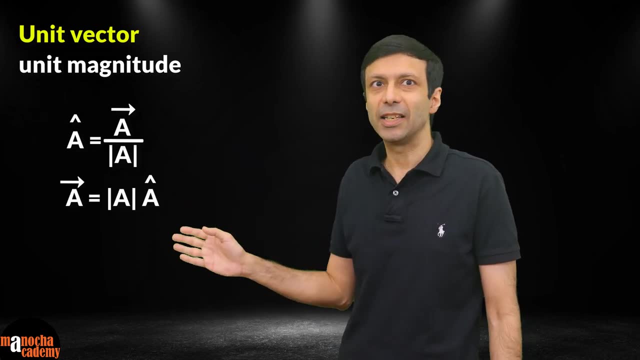 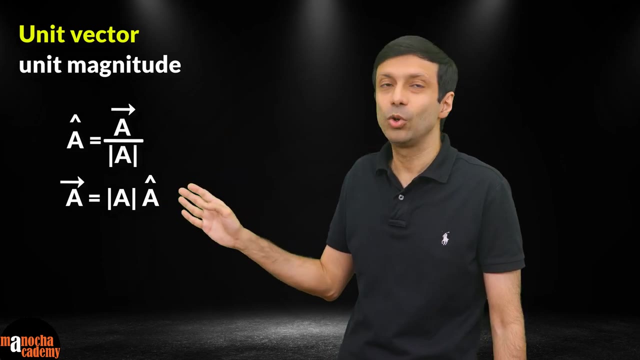 Unit vector is called A caret, A hat or A cap. Now, rearranging the equation, we can write any vector as its magnitude times the unit vector in the same direction. So the vector A is going to be the magnitude of A times the unit vector A hat. 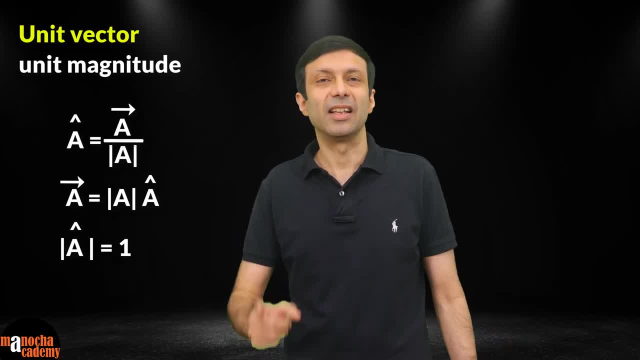 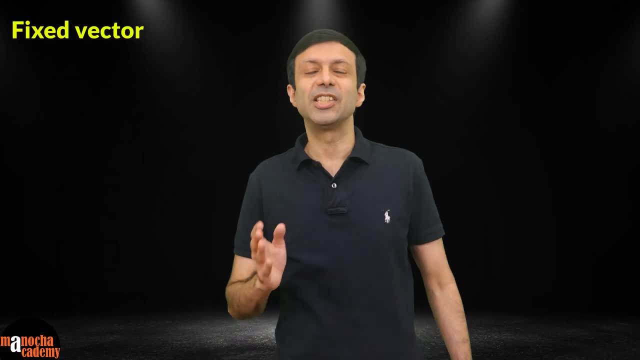 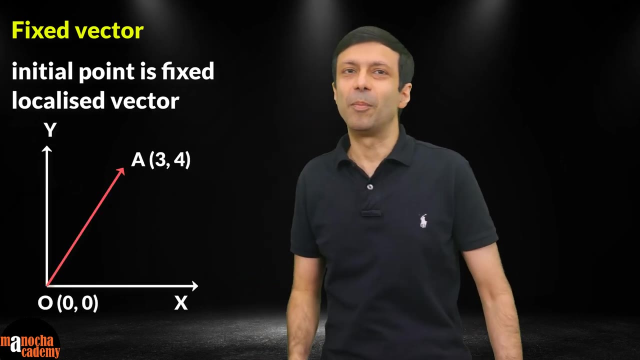 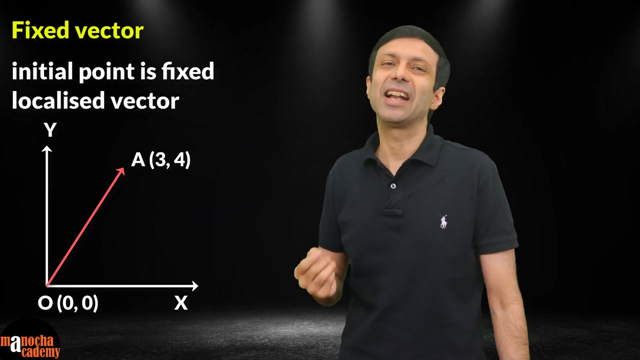 Note that the magnitude of the unit vector is unity, that is 1.. But the unit vector has no units or dimensions. Fixed vector is a vector whose initial point is fixed. It is also called a localized vector. For example, the position vector of a particle is a fixed vector since its initial point is fixed at the origin. 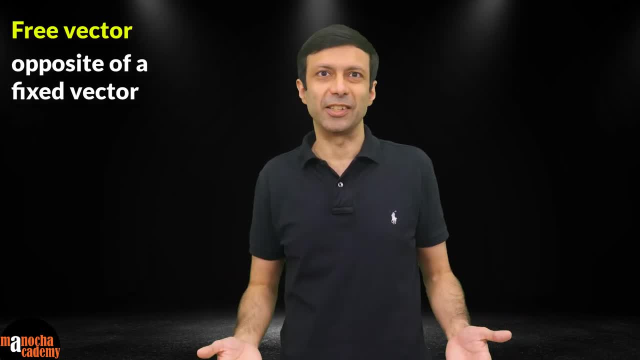 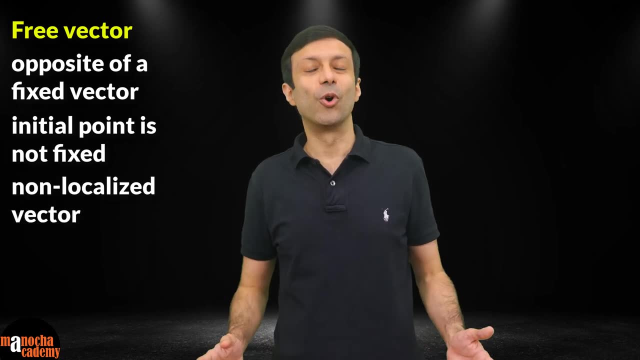 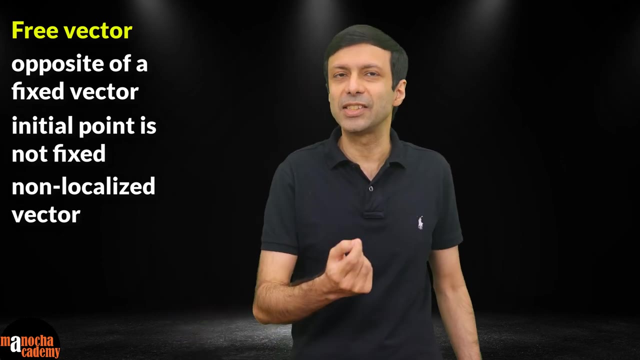 Free vector is the opposite of a fixed vector. Free vector is a vector whose initial point is not fixed. It is also called a non-localized vector. For example, force vector is a free vector. It does not have any fixed initial point. 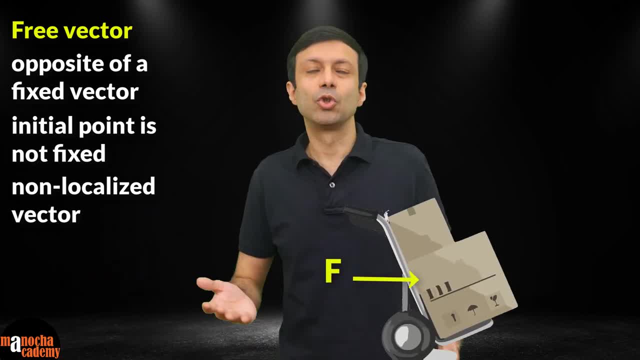 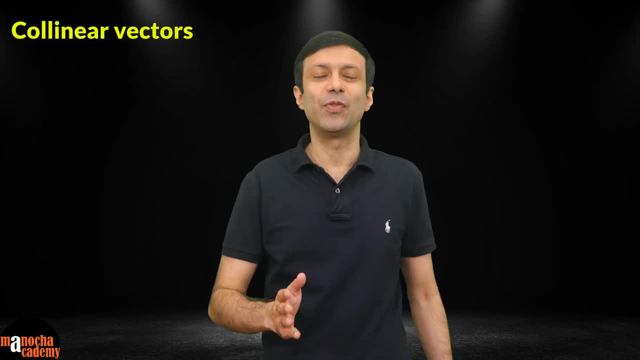 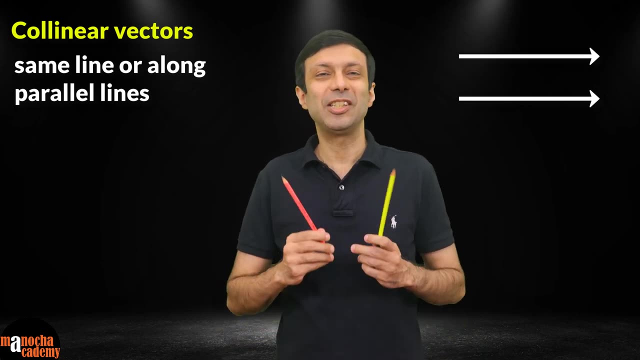 Because the force can be applied at any point right, So the force vector can move around. So that's why it is called a free vector. Collinear vectors are those vectors that act along the same line or along parallel lines. I am going to use these two pencils to represent vectors. 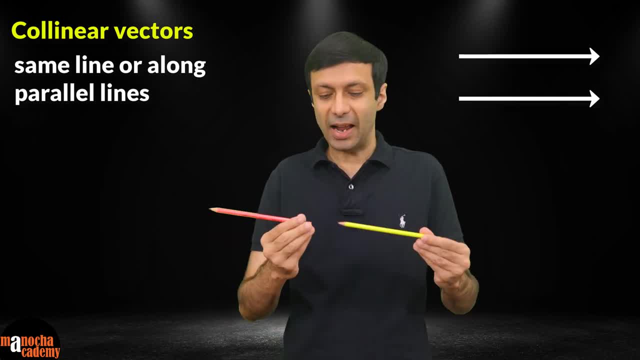 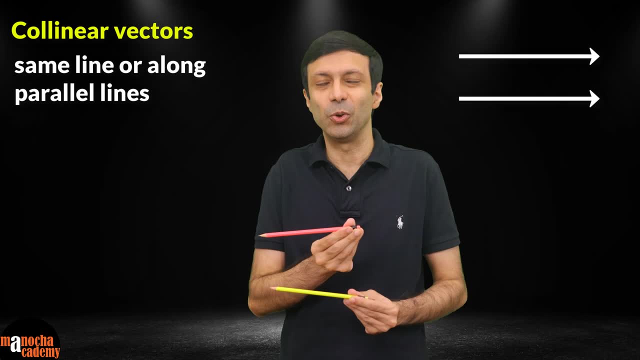 So when will they be collinear vectors If they are acting along the same line, like this, or along parallel lines? So see, these two are parallel to each other, So they are collinear vectors. The two collinear vectors that have the same direction are also called parallel vectors. 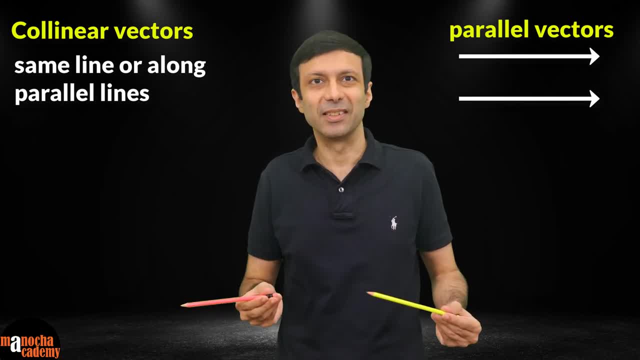 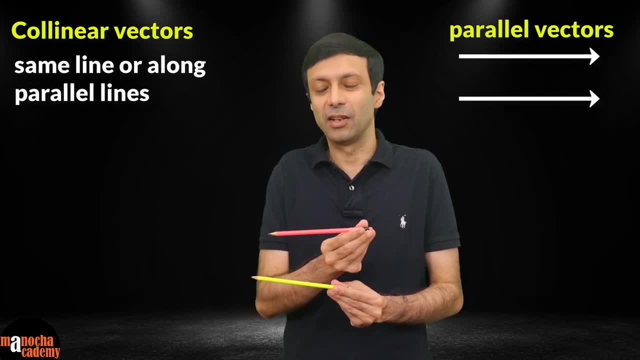 Now, what is the angle between the parallel vectors? Can you guys tell me? So, if you look at these two parallel vectors, can you see The angle is 0 degrees, which will be more obvious if you bring them together like this. 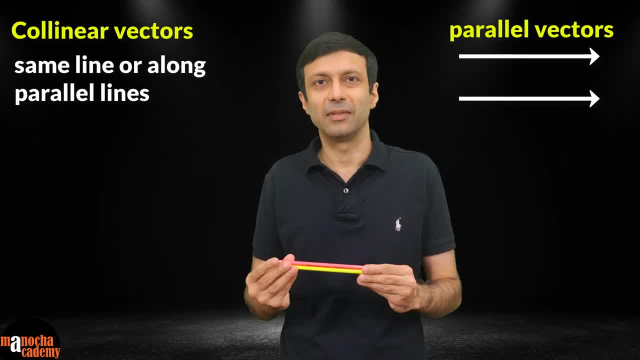 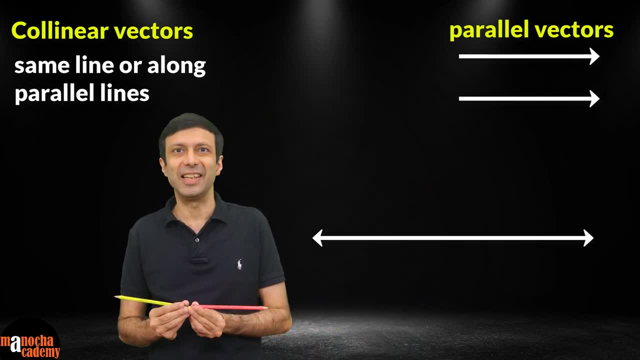 So if they are along the same line the angle is going to be 0 degrees. Two collinear vectors having opposite direction. so when they are placed like this, are called unlike or anti-parallel vectors. And what is the angle between the anti-parallel vectors here? 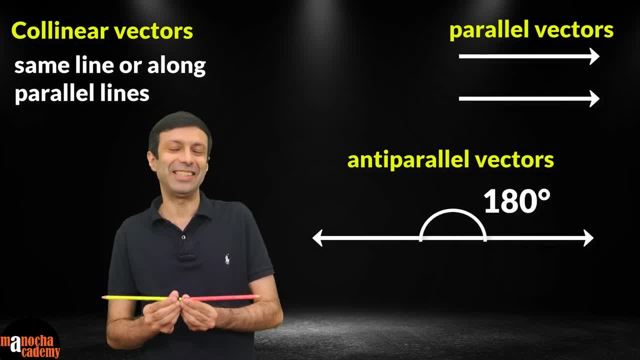 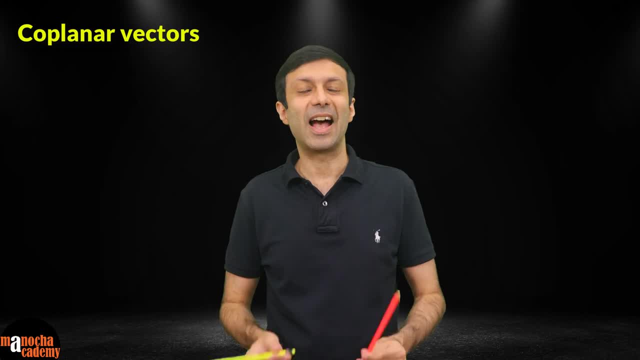 That's right. It's going to be 180 degrees here. So these are anti-parallel vectors. Coplanar vectors are vectors that act along the same plane, So if you have two vectors like this, they are lying along this same plane. 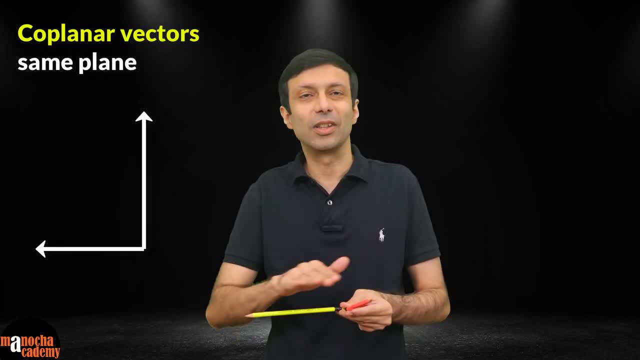 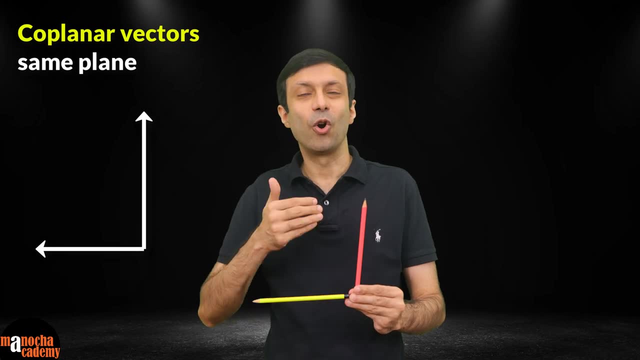 Or if the two vectors are like this: they are lying along the same plane or same surface. So let's say we have the two vectors like these. these will be called coplanar vectors. They are lying in the xy plane, So you can imagine a xy plane here. 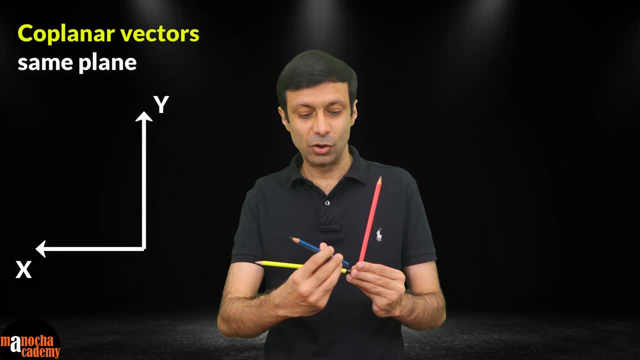 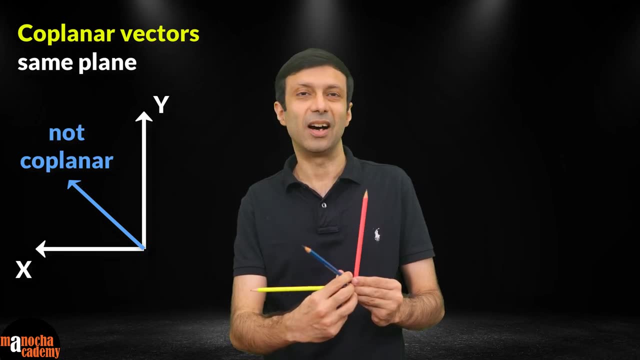 But if you have a third vector which is not lying in the same plane, a vector like this, then this vector is not coplanar with the other vectors. So coplanar vectors means it will also have to be like this. 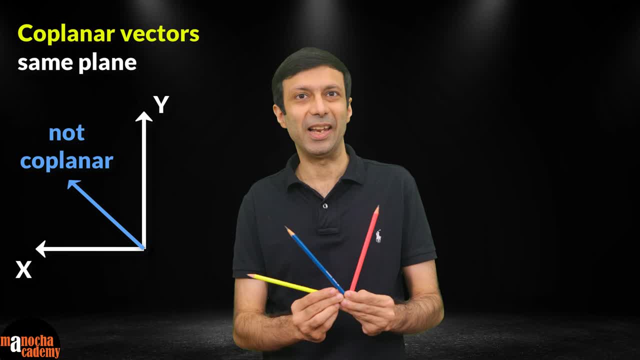 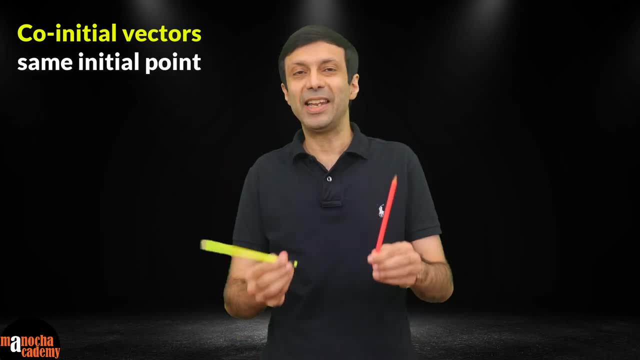 And these are see lying on the same plane here. Co-initial vectors are those vectors that have the same initial point. So if I take these two vectors, when will they be co-initial? When they have the same initial point, like this: 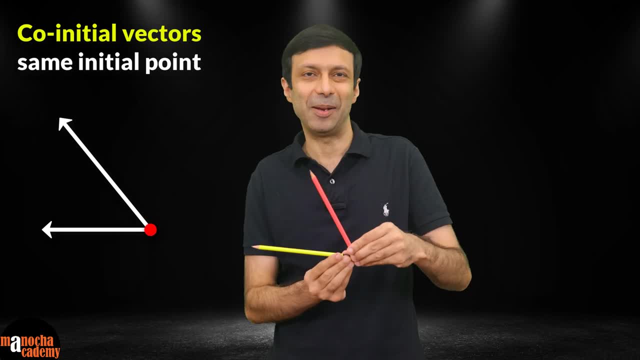 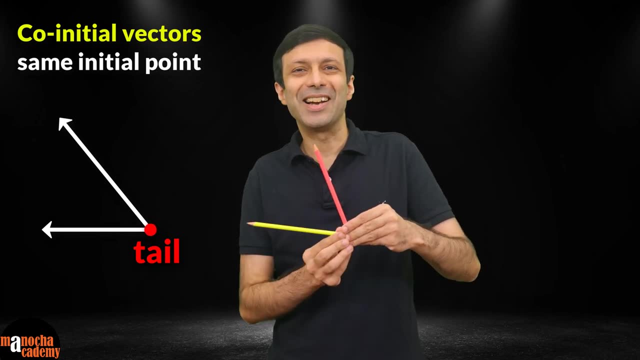 The starting point of these vectors is the same And remember, the starting point is called the tail of the vector. So, as you can see, the two tails are touching each other at the same point, So they are called co-initial vectors. 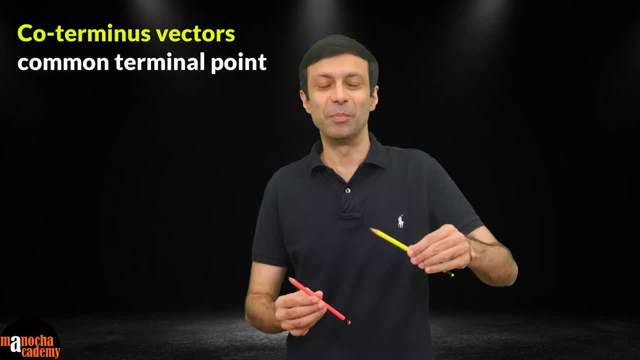 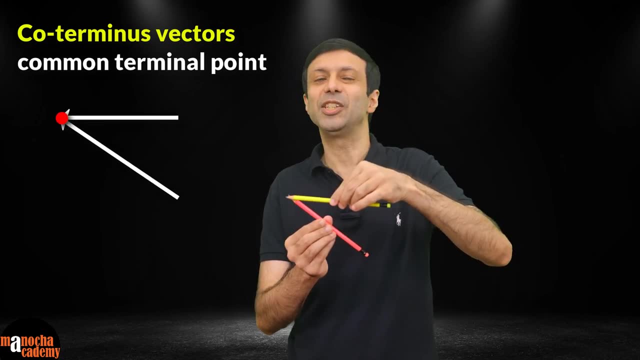 Co-terminus vectors are vectors having a common terminal point. So if you have two vectors, if they have the same terminal point, that is, the ending point is same. these vectors are called co-terminus vectors And remember, the ending point of the vector is called head. 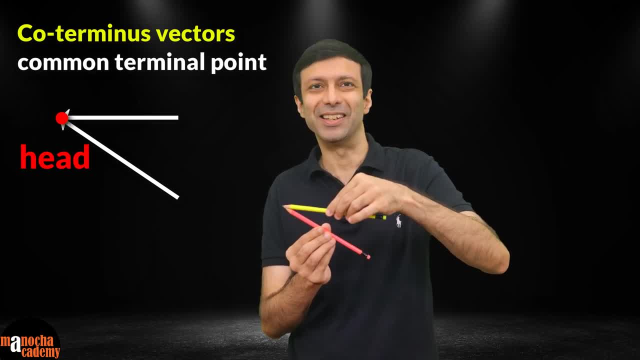 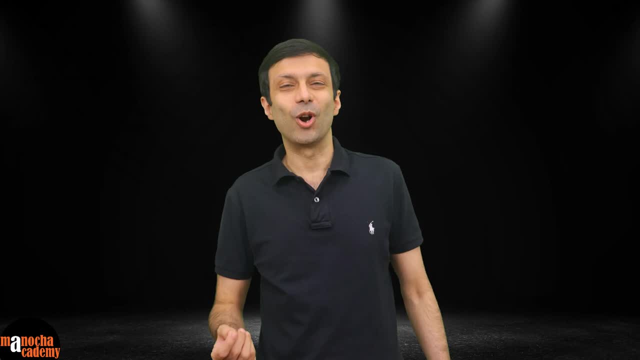 So we can say: the two heads of the two vectors are meeting here And these are co-terminus vectors. Now let's talk about a very special vector, which is called the zero vector. You might be thinking: why are we talking about a zero vector? 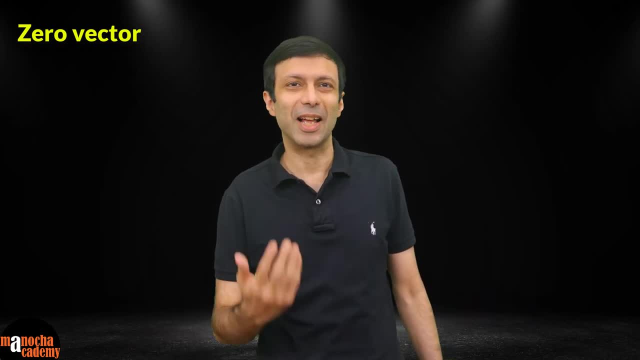 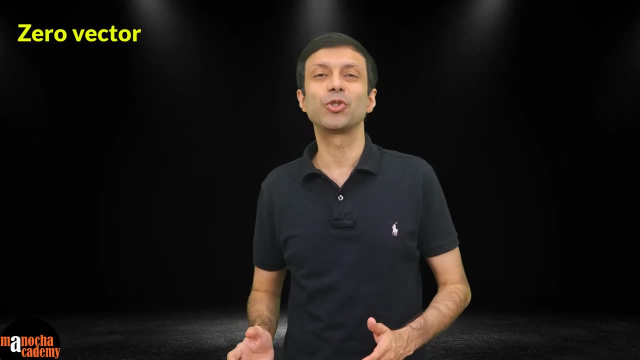 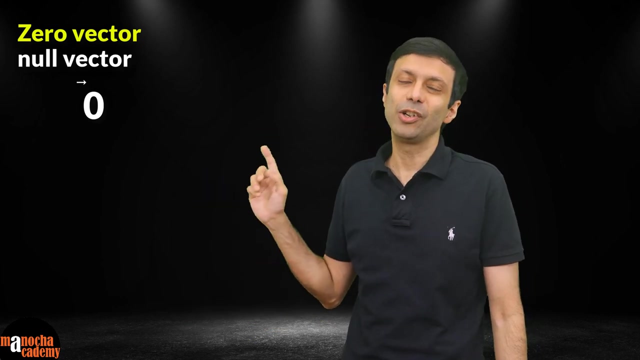 Just like the number zero is very important in mathematics, similarly zero vector is a very important vector. The zero vector is also known as a null vector. The zero vector is typically denoted as zero with an arrow on top of it. Now, zero vector is a vector. 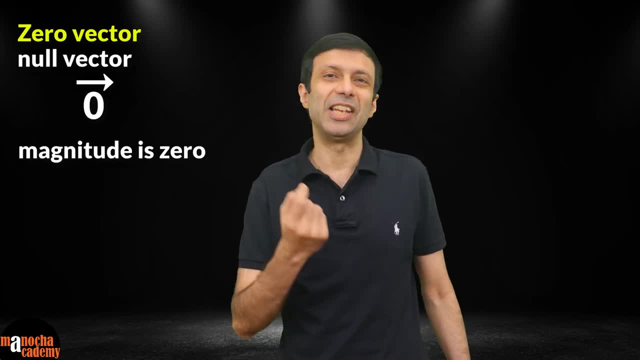 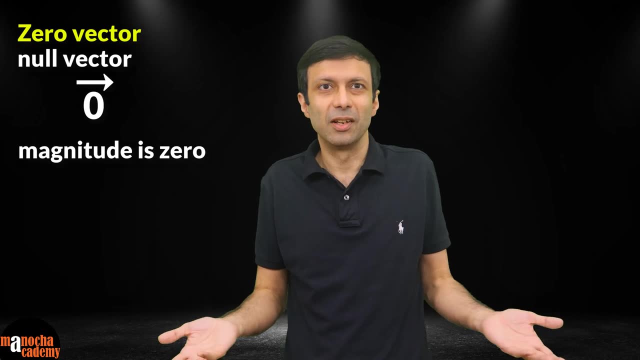 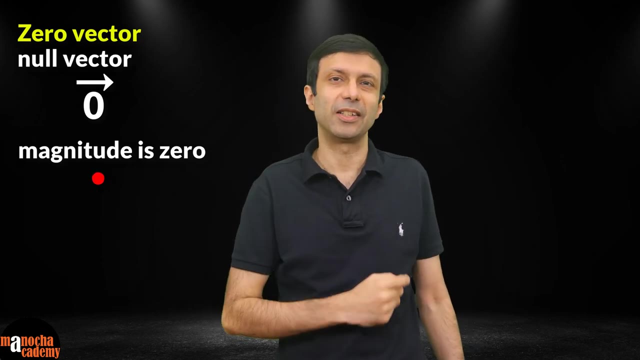 whose magnitude or length is zero. A zero vector does not have a specific direction, or we say it has an arbitrary direction because it's a zero vector. so where will it point to? It is often shown as a point or a dot in the vector diagrams. 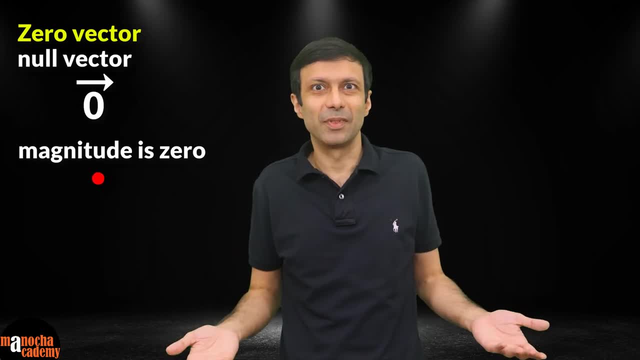 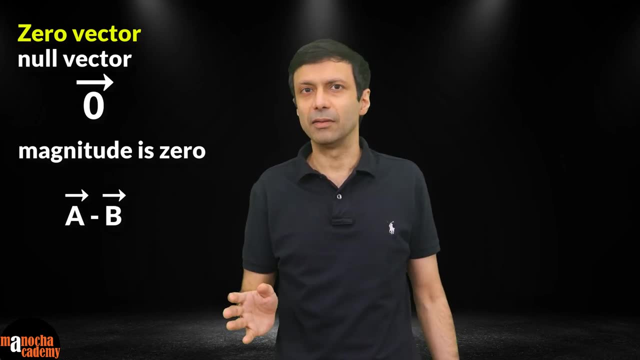 because it doesn't point anywhere. Now why do we need a zero vector? Let's say you have two equal vectors, A and B. So can you tell me what is A minus B? It will be zero, right, But when you subtract two vectors, 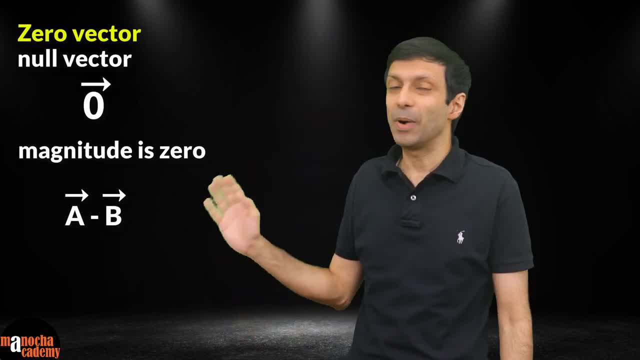 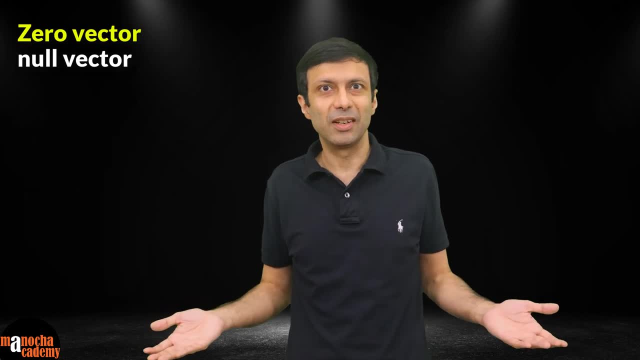 you should also get a vector. That is why A minus B is going to be equal to the zero vector. What are some other examples where the zero vector can be used? Let's say a particle lies on the origin, Then its position vector is a zero vector. 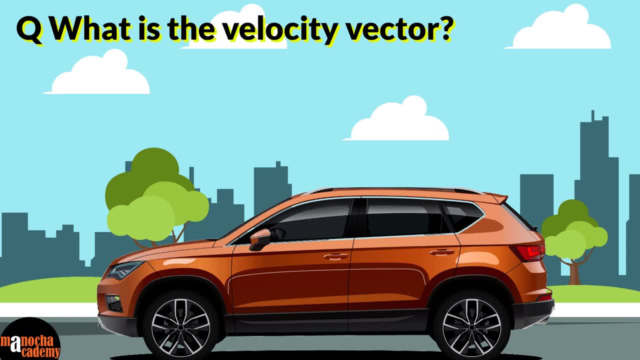 Similarly, what will be the velocity vector of a stationary object that is, an object at rest? That's right. Once again, it's going to be a zero vector because it is at rest. So zero vector is important and it has practical applications. 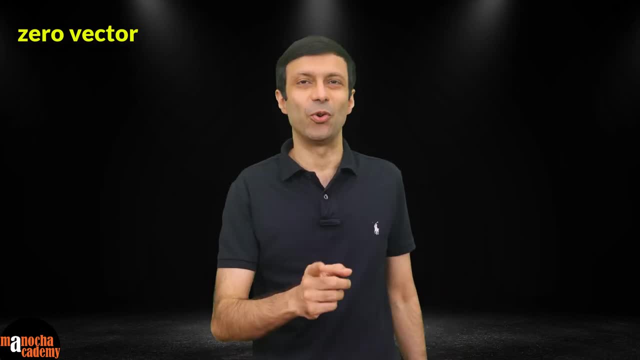 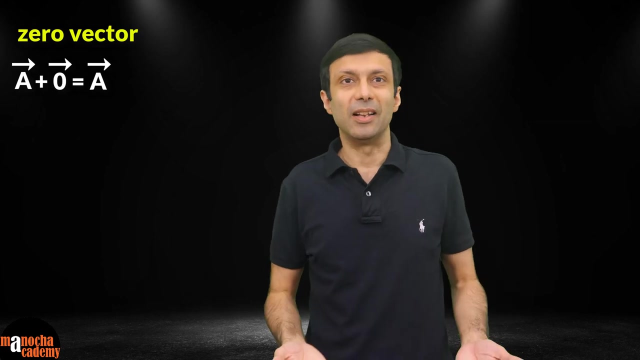 Let's discuss some mathematical properties of the zero vector. When you add the zero vector to any other vector, the result is the original vector itself. So for any vector, A, A plus the zero vector equals A. Similarly A minus the zero vector. 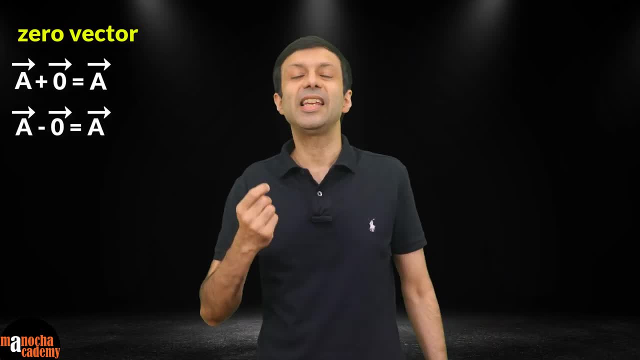 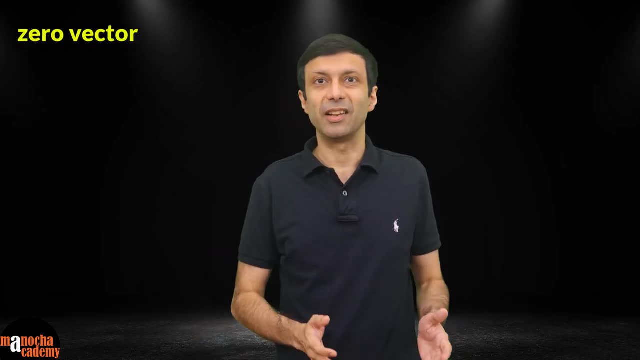 is also equal to A. So zero vector is the additive identity for vectors. Now when you multiply a real number by a zero vector, it results in the zero vector. So if k is the real number, k times the zero vector. 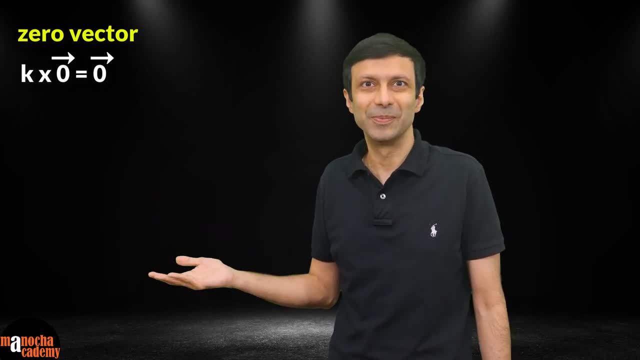 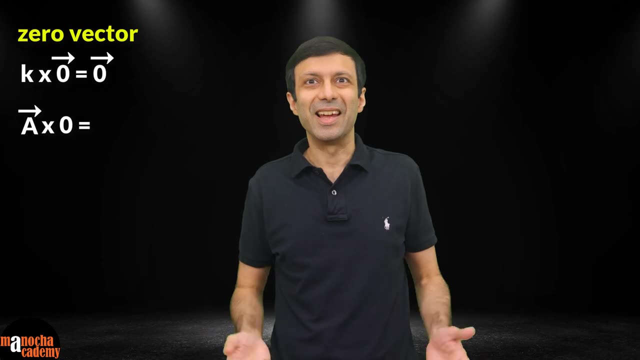 equals the zero vector, because you are multiplying it with the zero vector. Now, if you take any vector, let's say A, and you multiply it by the number zero, what do you get? That's right, You will get the zero vector. 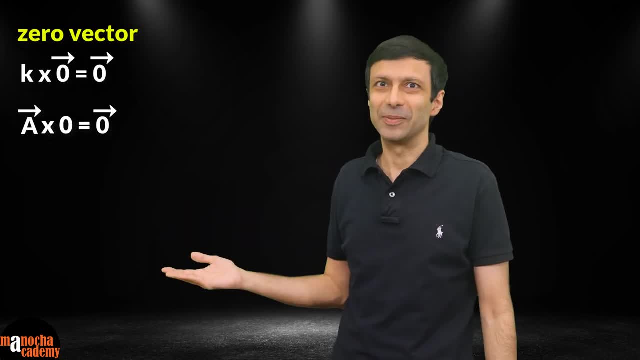 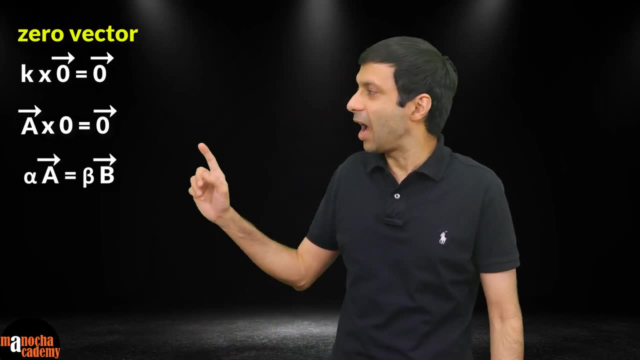 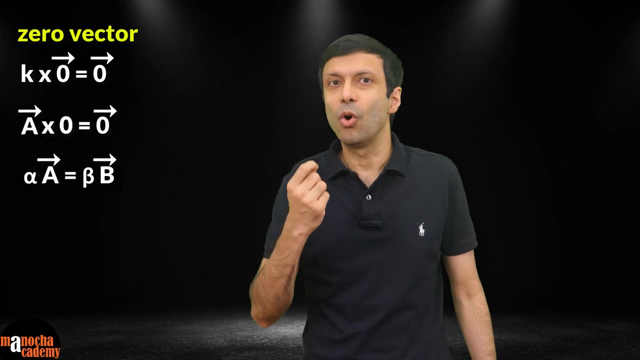 So zero times the vector A equals the zero vector. If alpha and beta are two different, non-zero real numbers and alpha times the vector A equals beta times the vector B, then this relation can hold only if A and B are both zero vectors, because alpha and beta are different numbers. 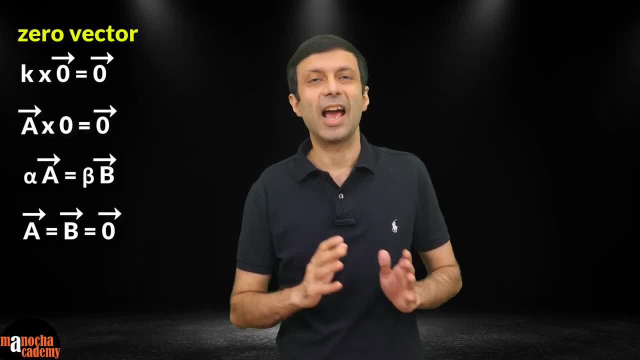 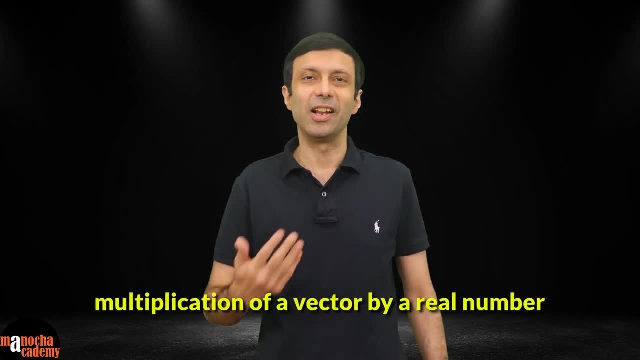 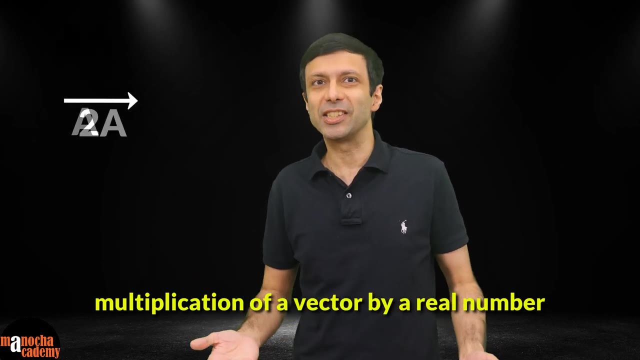 So the equality will hold only if A and B are both zero vectors. The last thing we will look at is the multiplication of a vector by a real number. For example, if you multiply a vector A with 2, this results in a new vector, 2A. 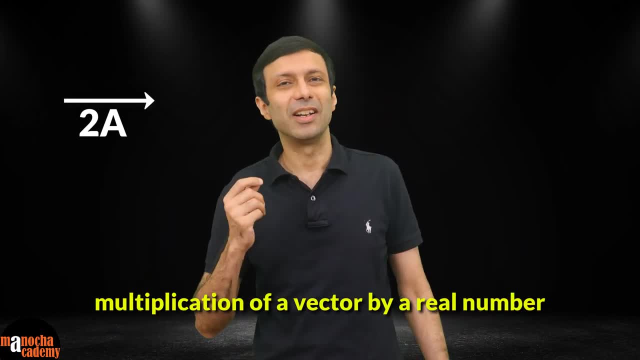 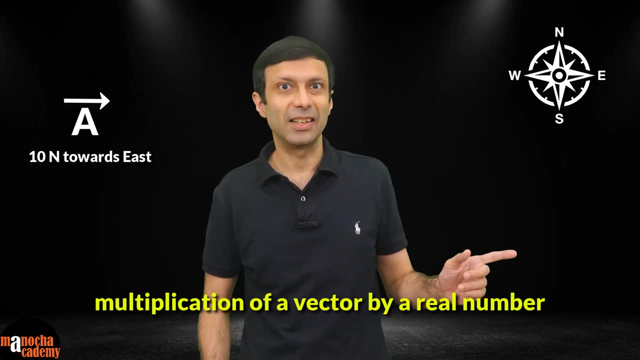 That is double in magnitude but it has the same direction. So if A was a force vector representing a force of 10 N towards the east, then 2A is a force vector representing a force of 20 N. that is double the magnitude. 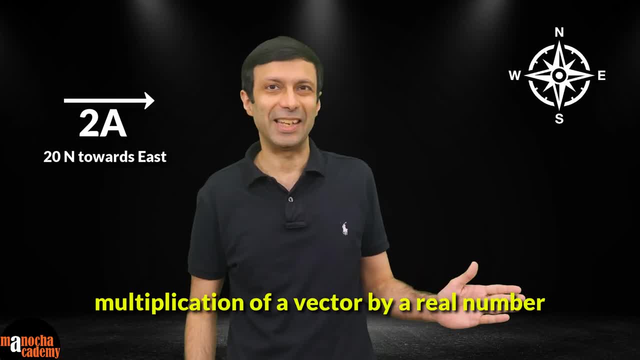 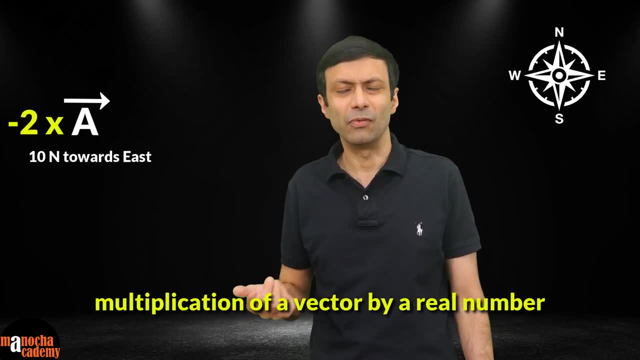 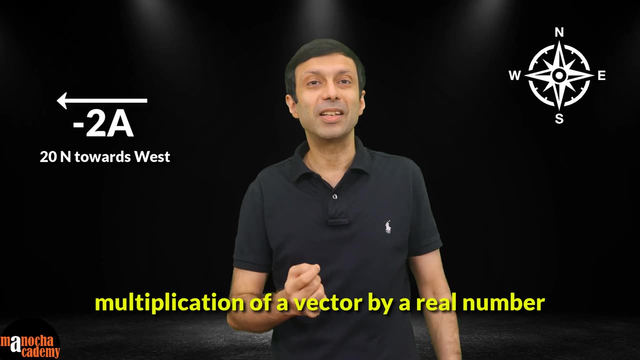 but in the same direction, that is, towards the east. But what will happen if we multiply the vector A with minus 2? Will it give us the same answer? No, It will give us a force of magnitude 20 N, but in the opposite direction. 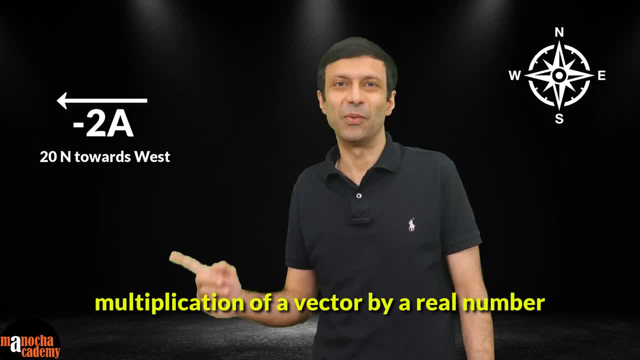 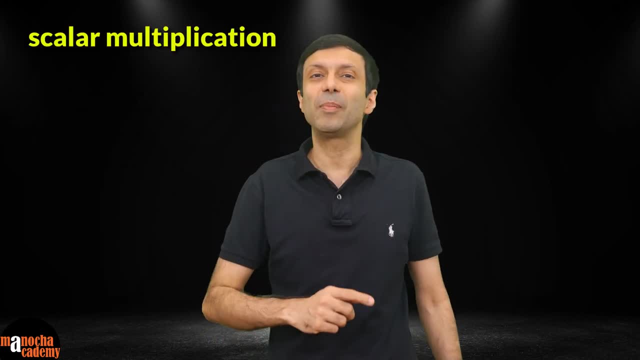 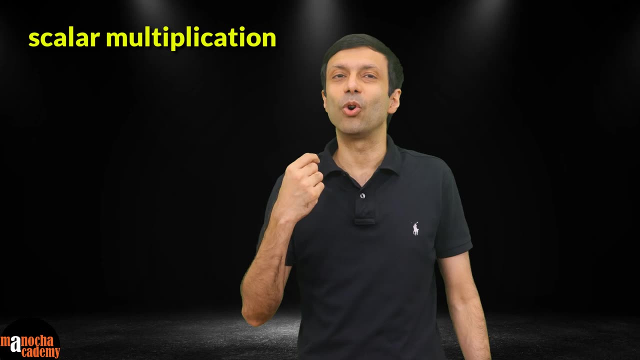 because there is a minus sign, that is, the force will be towards the west. So multiplying a vector by a real number is known as scalar multiplication. as we are multiplying the vector with a number which is a scalar, It results in a new vector that is related to the original vector.